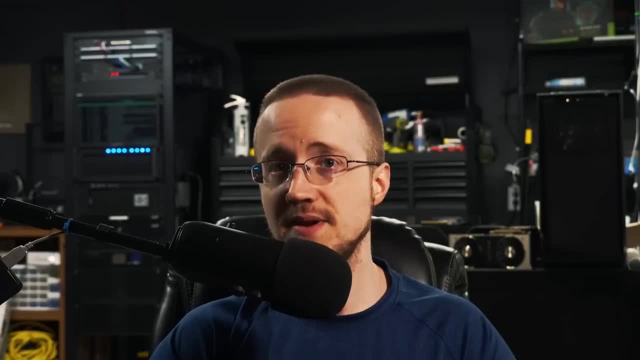 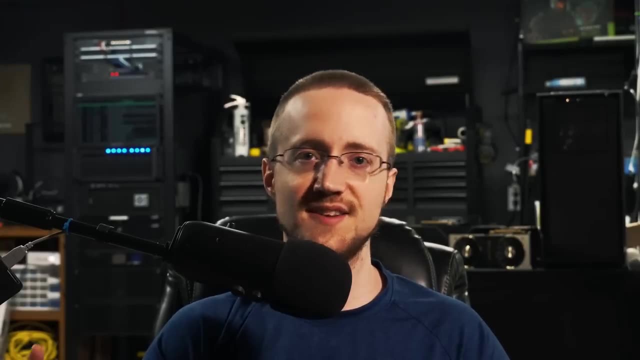 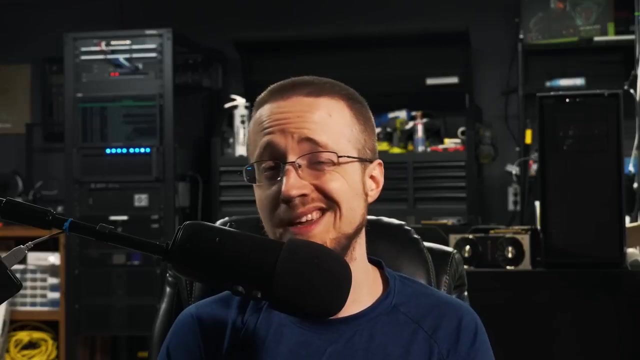 needing a mere 10-ish gigabytes of memory at 8-bit. The 40 billion parameter variant can be a little more challenging, wanting more like 45 to 55 gigabytes at 8-bit and 100 plus at 16, depending on context length. You can feel free to run these locally, even on CPU and RAM. 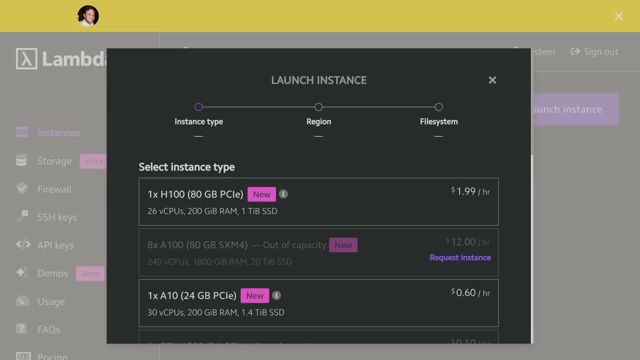 if you want, but I would personally suggest Lambda for the $2 an hour H180 gigabyte card. but they don't pay me to say that, It's just a fact. they are the best right now in terms of price to performance. on cloud hosting, Getting set up to actually run the Falcon models is most likely. 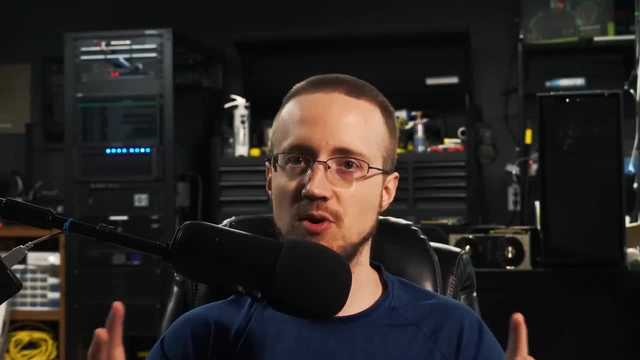 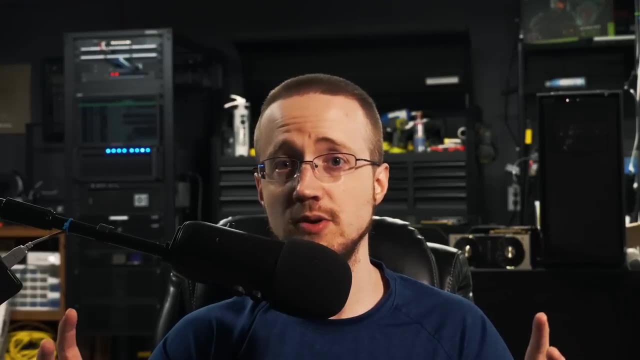 going to be just upgrading to Torch 2.0, since I imagine most people are still on 1.x in some form. In the description of this video, I will have a link to my GitHub with all relevant code and snippets, including the install shell script that I personally used with Lambda to get things rolling. 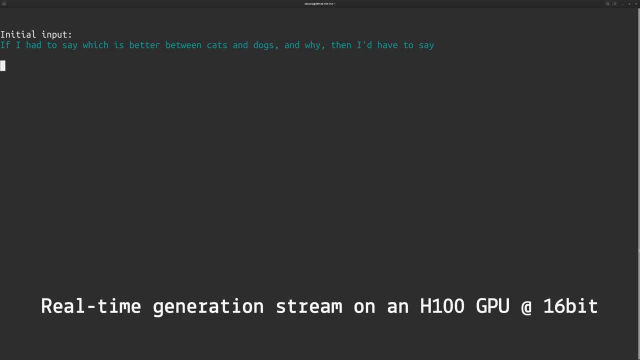 but this would work on AWS or other platforms as well, even locally. From here, we can check out a basic example of how to run the Falcon model. I'm going to show you how to do that in just a few moments. Here's an example of Falcon 40B's performance and quality, And in this case, 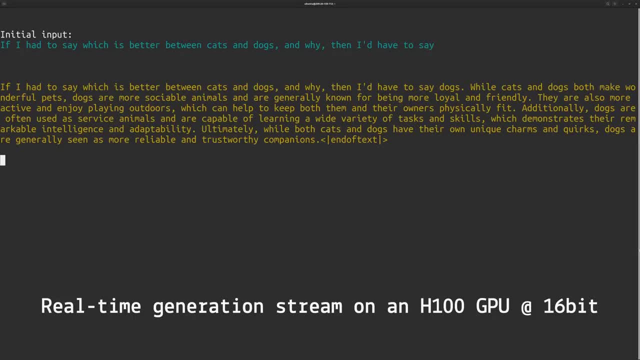 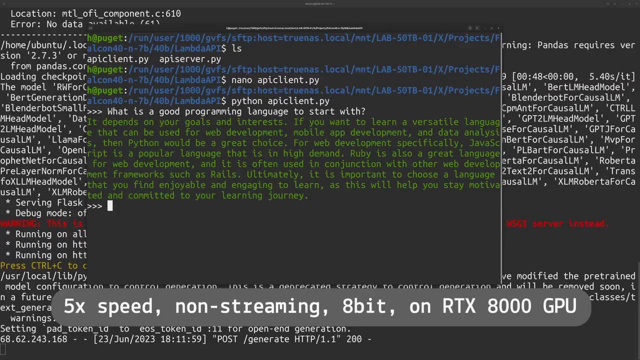 it's just continuing a thought. Of course, though, this is an instruct model, which can be more geared towards things like instructions or a conversation, So let's try that. As you can see already, the Falcon model has a pretty good grasp of the natural language. 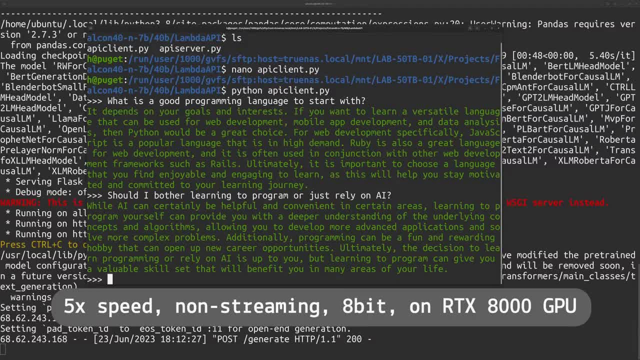 It's really quite interesting to me how fast this bar to be impressed by large language models has moved, since chat GPUs have become the most common language model in the first place. This is probably the most interesting example of Falcon's performance and quality, And in this 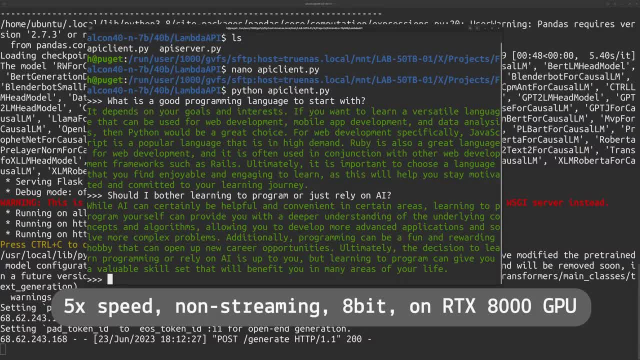 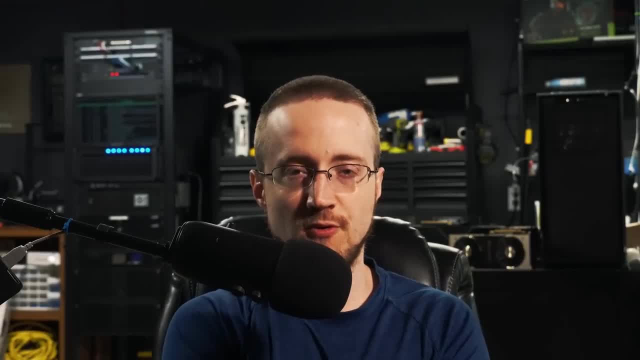 case, it's just continuing a thought. Of course, though, this is an instruct model which can be more hit the scene. late last year, like a year ago, just a year ago, this alone would have been just huge like this, just just falcon 40b's performance right now, like would have been. uh. 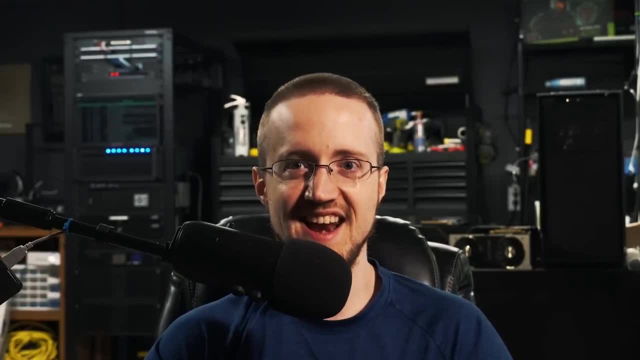 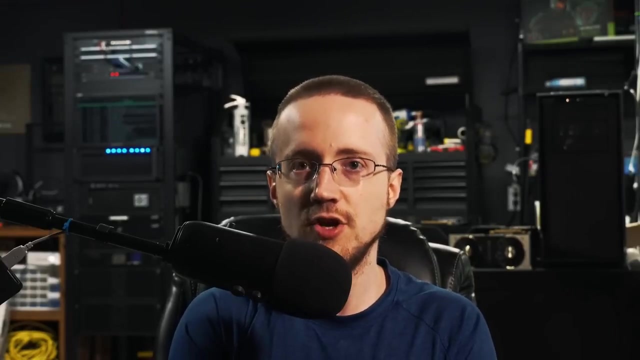 just massive, huge breaking news. and when chat gpt came out, it was and suddenly we, just we just happened. we just live in a world now where we have these models that can speak and generate text, as if we're speaking to a human, or another human is writing to us and it's a. it's good enough to. 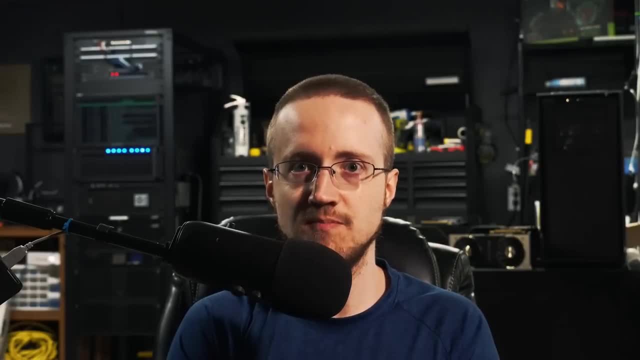 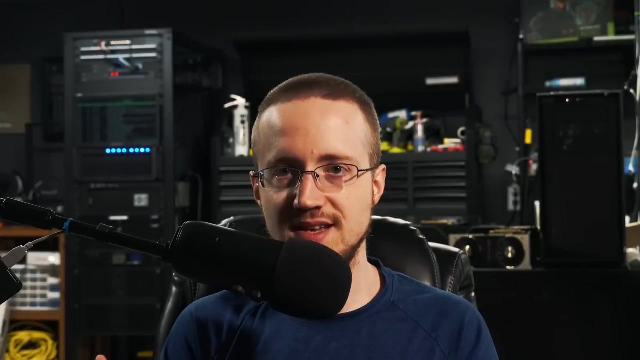 convince other people that it is another human, indeed writing to us, and i think what makes falcon and falcon 40b especially huge right now is, rather than needing to run all of your queries through open ai, you can just download and run falcon on your own, or you can fine-tune it further. it's 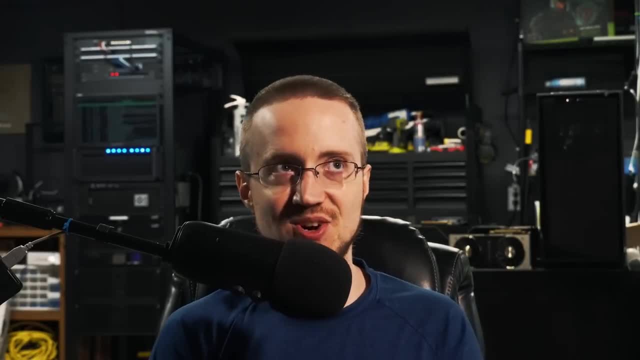 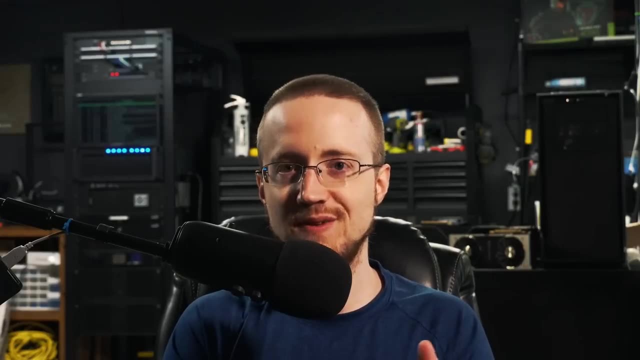 yours to do with as you please, and it's just crazy to me the the progress that we've made in just one year and a half. it's just crazy to me the the progress that we've made in just one year and a one year in ai and what's actually available to people to use, like right now, in software. 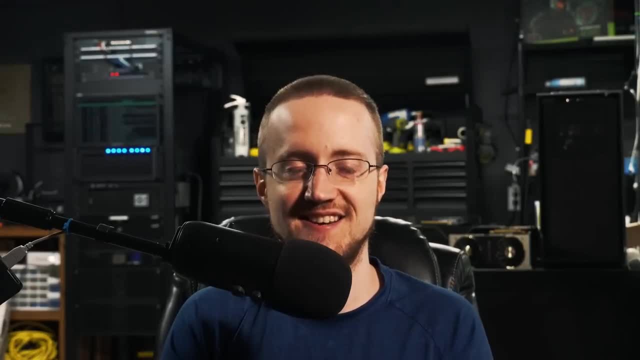 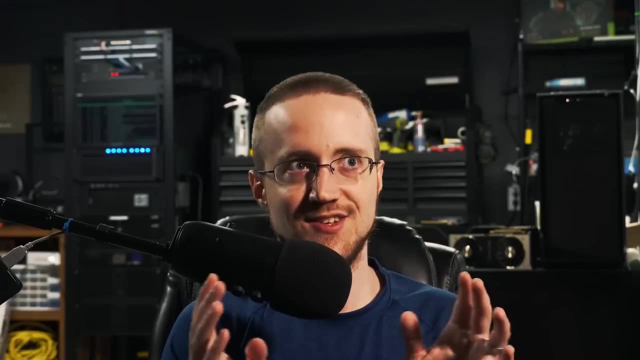 development and and just the, just an ai that is available to you. and now ai that is available, literally that you could just download, it's yours, you do whatever you want with it from here. that's just insane. it's just insane, as you'll soon see in some of these examples, i actually 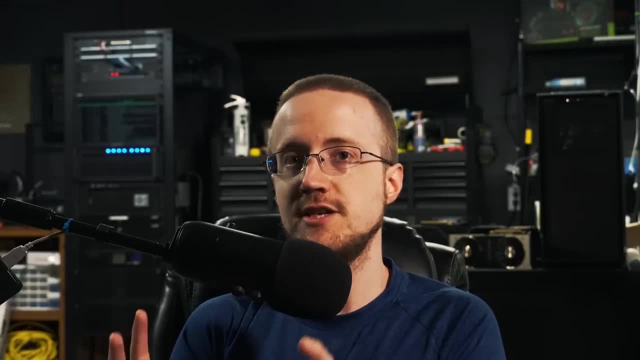 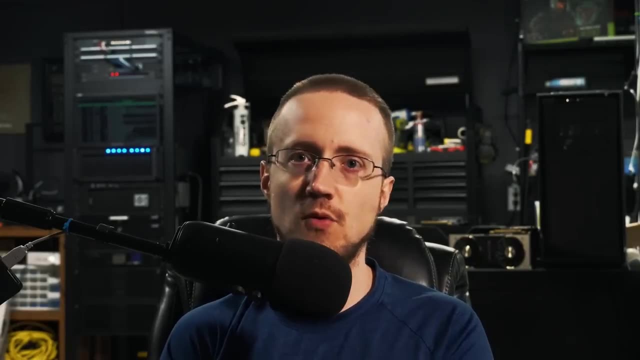 think falcon 40b is very comparable to chat gpt's base model, the gp or gpt 3.5. uh, it's a little inferior to gpt 4, but we'll talk a little bit more about some reasons why i think that is. 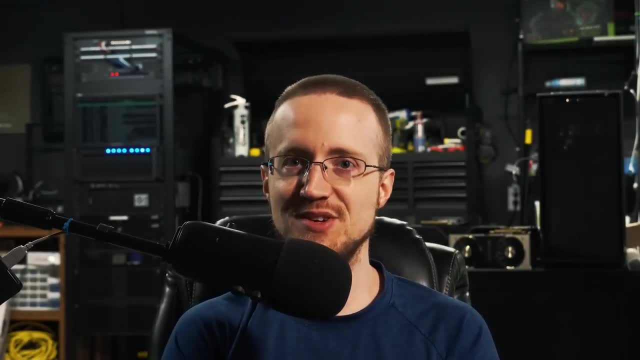 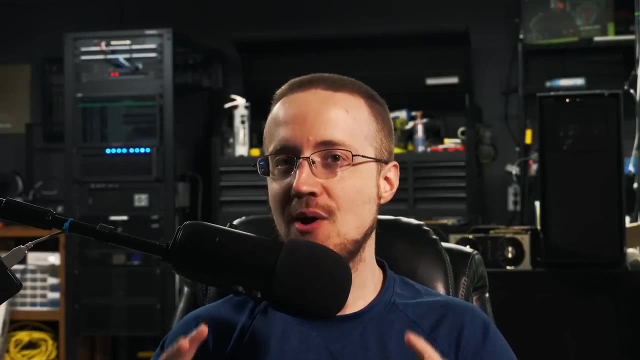 but also it's just a vastly smaller model than gpt 4, but i think we actually could probably eke out a lot more performance than just what the model itself right now is outputting. so how intelligent is falcon? for all these examples, i'm going to just use the falcon 40b instruct. 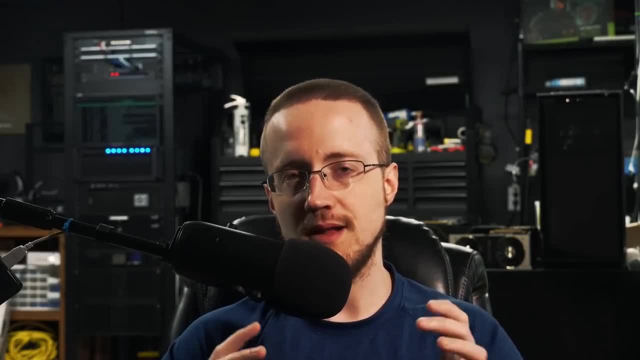 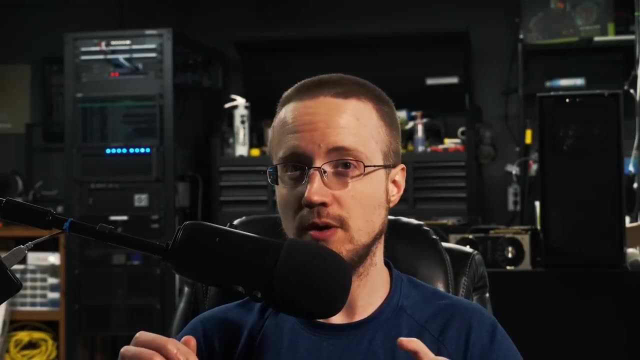 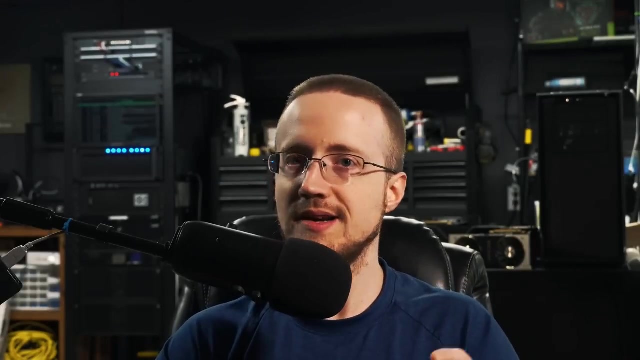 model. from my very brief testing, i would likely classify falcon 7b as best suited really for the, for either like few shot learning examples or even likely as a model that you'd further fine-tune to a very something more specific, whereas falcon 40b, especially that instruct variant, is much more. 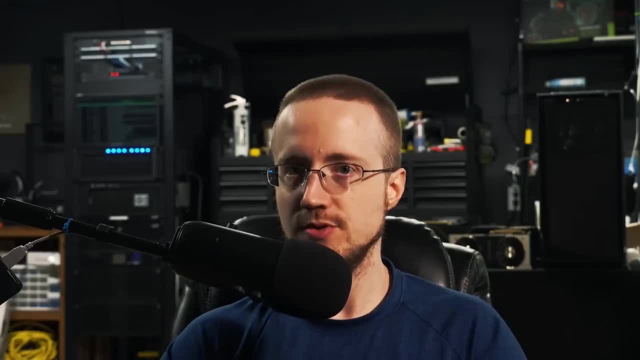 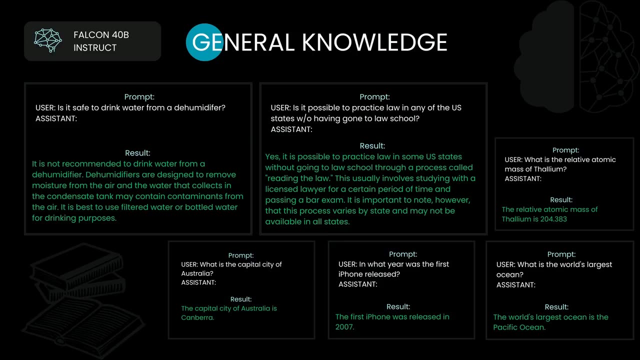 suitable for just general use and working right out of the box. to start some fairly random general knowledge questions. here i'm showing what the initial prompt input was and then the results. to the best of my knowledge these are all accurate and good answers from falcon 40b here. as you can see, i used a sort of format in my prompt to suggest. 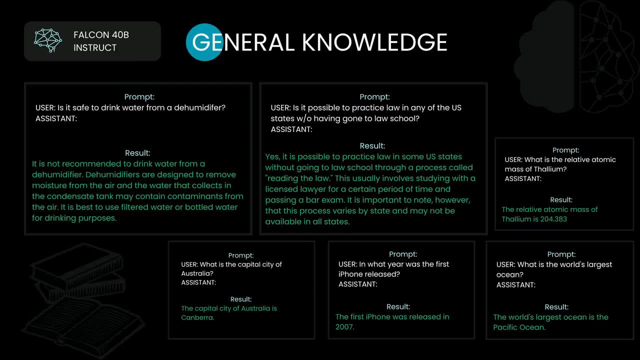 a sort of conversation between a user and an assistant. these names do not need to be this way or the same, or even used at all. this model is extremely open and general purpose. you don't even need there to be like one to one, like user then assistant, then user then assistant, you can have. 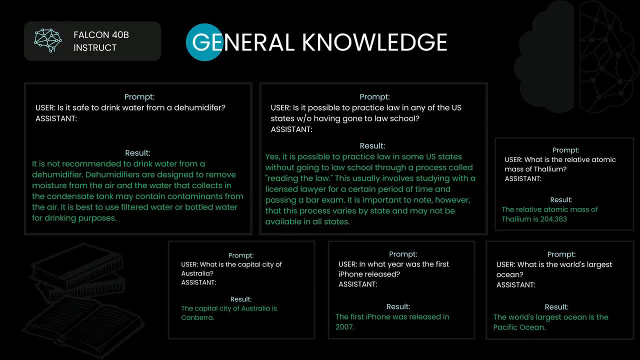 something like user assistant, assistant, assistant, like. i'll show example of that later too, but there's, the possibilities here are very, very open. so here, though, i do particularly like the question about practicing law without a law school degree in the united states, because most models get this wrong and and the question and answer itself can- 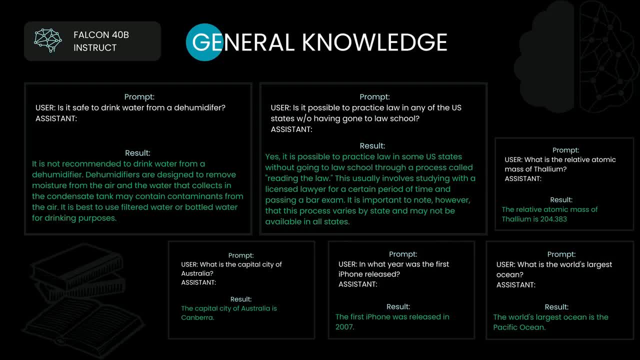 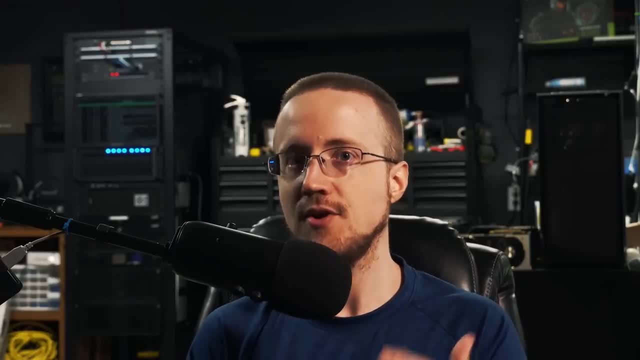 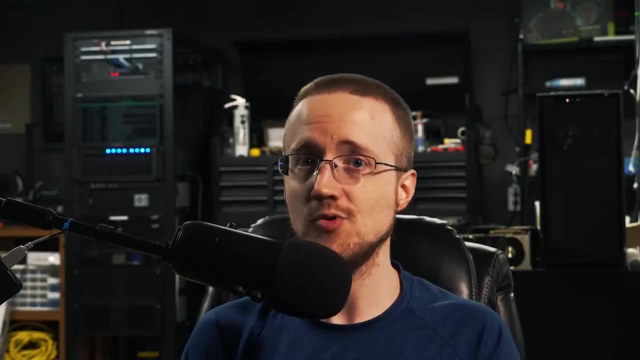 also speak towards potential uh, moderation and, after the fact, sort of censorship or just a bias towards safe answers if there are concerns about models saying incorrect or unsafe things. in general, highly professional fields like law and medicine carry a lot of risk if people who are uneducated 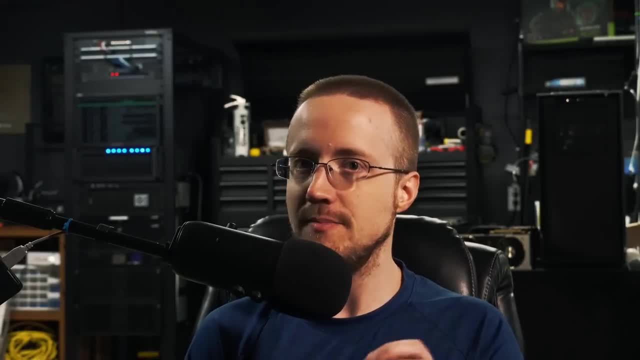 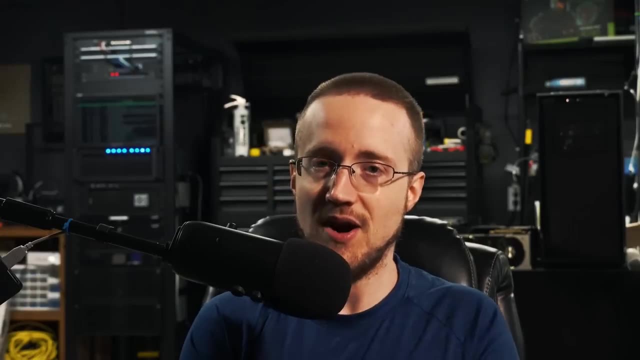 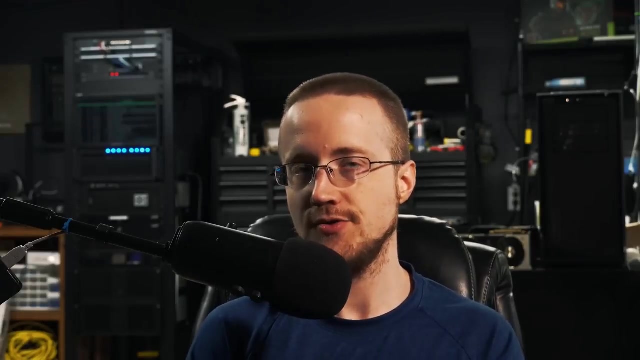 attempt to practice it. so a model is likely to be biased away from answering this question correctly, even though that is the truth that you can practice law in certain states without a law degree, if attempts are made to encourage or bias that model towards safe answers. so, for example, chat: 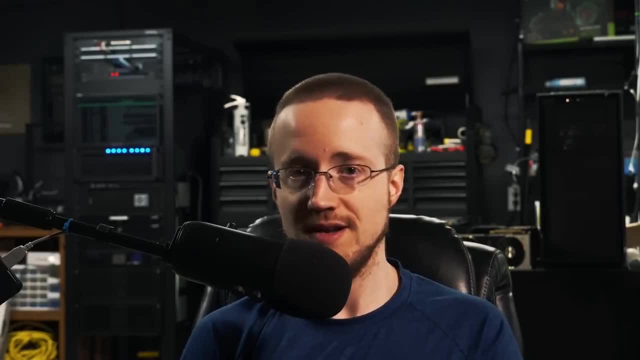 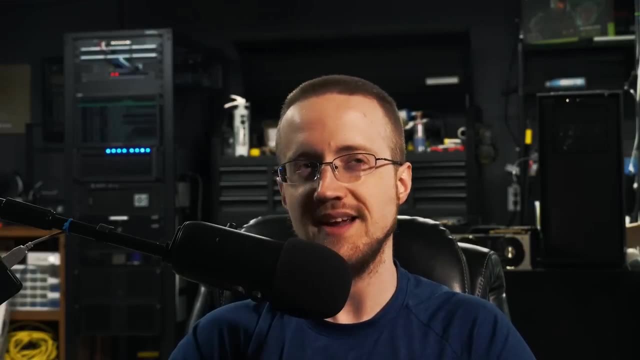 gpt with gpt 3.5 gets this wrong and says no, you cannot practice law in any state without a law degree. gpt 4.0 does act the same way, so i'm going to try to get this right, and i can't remember if it's always gotten this question right. 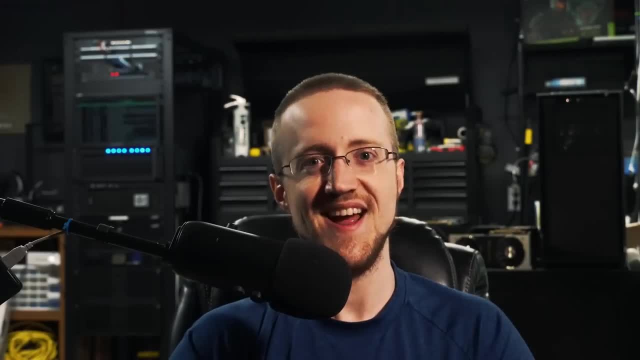 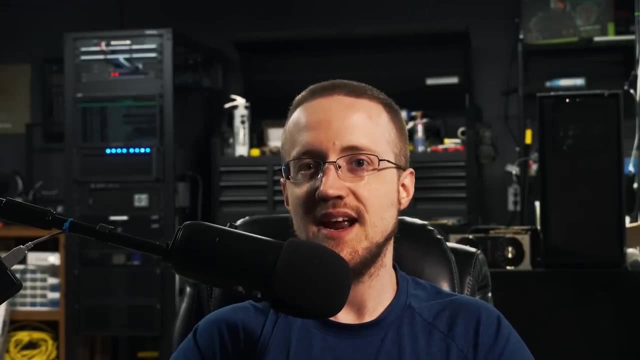 i want to say, if memory serves me, it didn't used to get this question right, um, but anyway, here it does, but now without multiple warnings and what i would call cyas. so it does seem that, at the very least, the potential risks in answering this question. 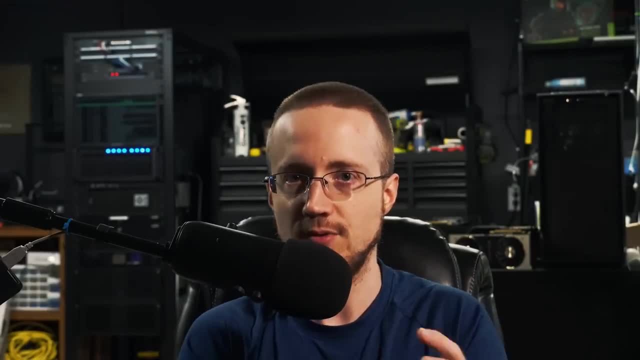 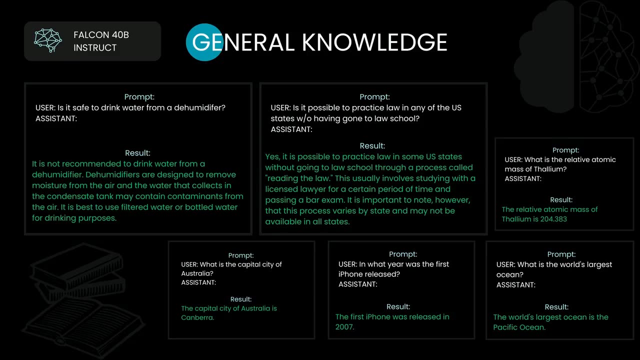 were identified by gpt 4.0, and then it's very careful in its response to you. now, beyond this question, all the answers indicate a wide range of accurate knowledge that you can tap into, from the of drinking dehumidifier water to the iphone's release date, to the atomic mass of thallium. 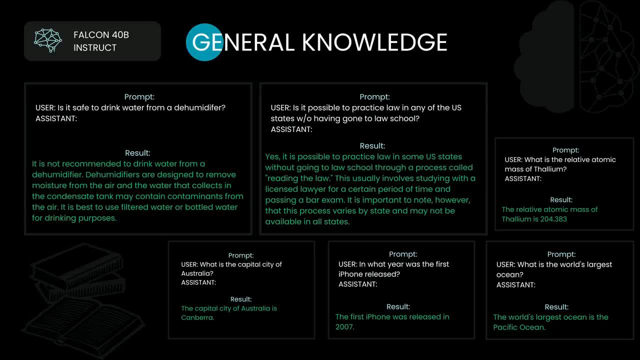 and so on. obviously, this is a terribly small sample size and i'm confident that we could find wrong answers generated by this model, but as a general purpose model, this is really surprisingly good for a mere 40 billion parameters, at least in my opinion. next up is the topic of math, an area 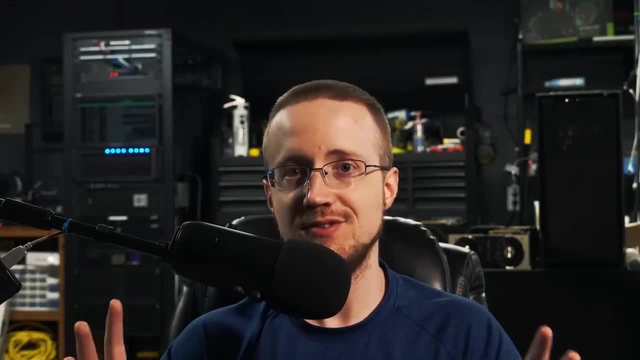 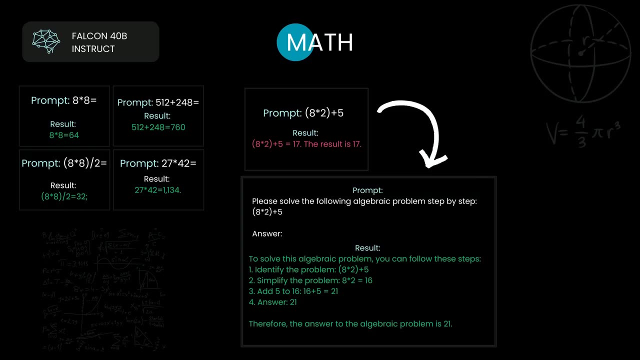 that gpt models tend to struggle significantly with due to the autoregressive nature of how they actually generate responses going always linearly. algebraic expressions are often calculated in like chunks and not necessarily in a linear order of the characters that are seen right. so large language models. 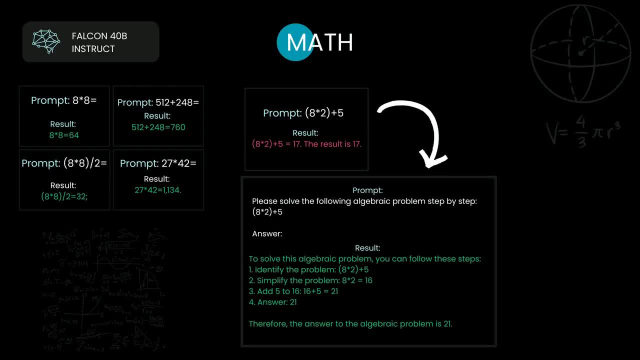 often struggle here. for simple math problems falcon 40b gets the correct answer. but as you complicate things with algebraic problems you can often find gpt models, including even gpt4 and gpt 3.5. they begin to struggle. chat gpt, especially for gpt4, uses something in the background. 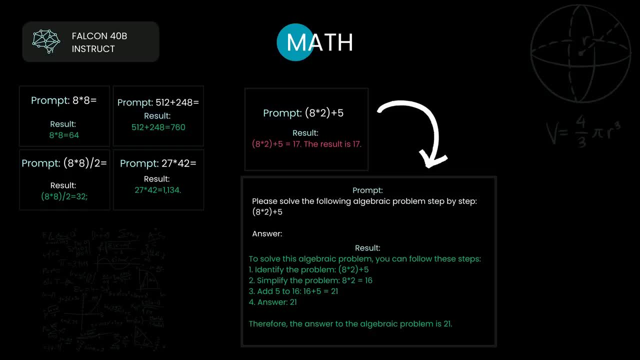 that will essentially convert your math prompts to show your work prompts. so where the the machine was, a, at least asked. i just want this answer. it is clearly detecting that it's a math problem and then being fed an additional- i think- prompt that is suggesting that, hey, please show your work. 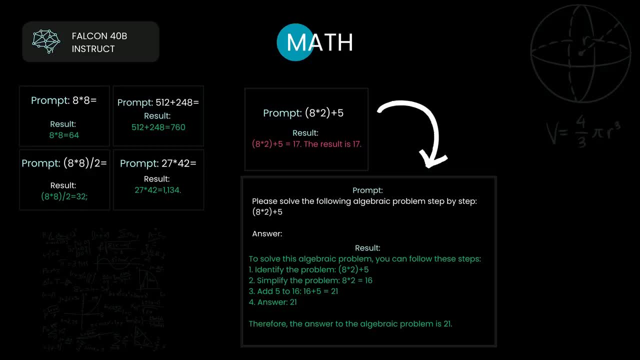 because this is a common trick to getting gpt models to correctly solve problems like this that are maybe not necessarily solved by thinking linearly, like if you need to kind of be able to bounce around. um, the way to do that is essentially asking it to show its work and the theory here. 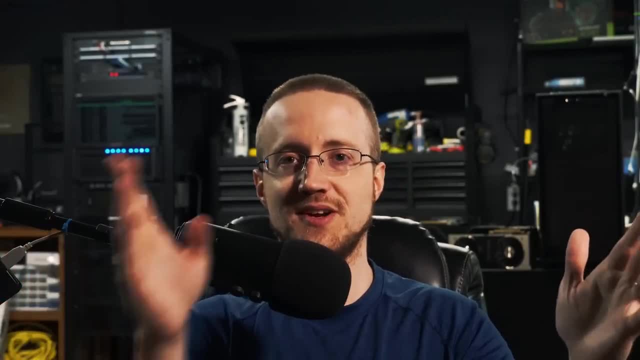 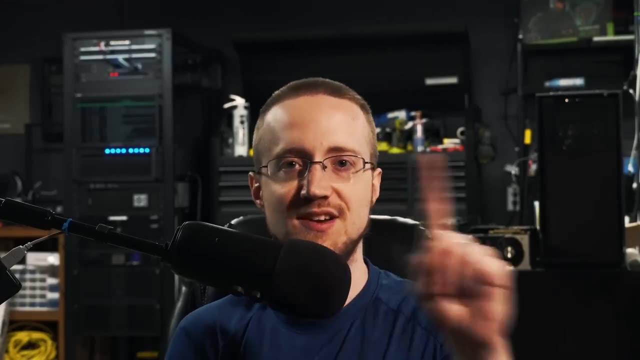 is just the more tokens that you give the model to kind of like think through a problem. that's like token is like brain power or something, and then it also allows it to think non-linearly now, whereas if you tell it just straight up, give me that answer and nothing more, it's probably going to. 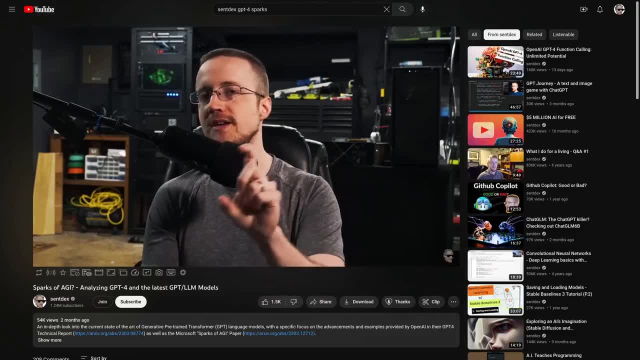 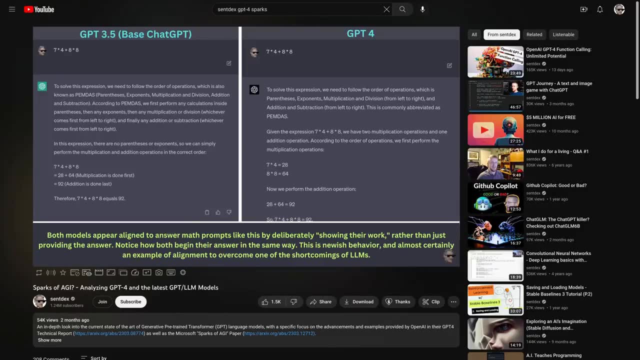 get it wrong. i also exemplified this example in my analyzing gpt4 video. i'll put a link to that video in the description. but here's a couple of friends from that where gpt 3.5 and gpt4 get this right nowadays, due to some gpt post processing or uh, you know just. 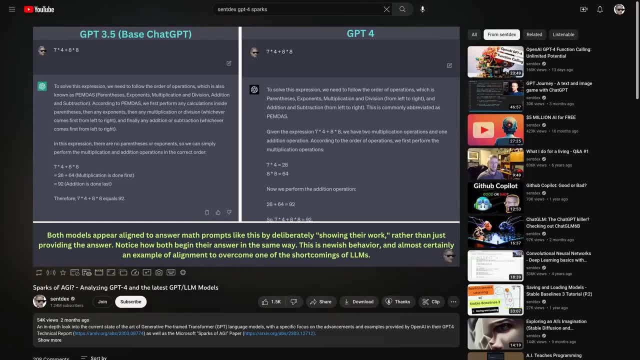 tricks that are being applied and actually gpt 3.5 got these questions, used to get these questions wrong and i actually think, using rbrms and other kind of heuristics and techniques and stuff that that open ai learned from gpt4. i think they just went back and applied them to gpt. 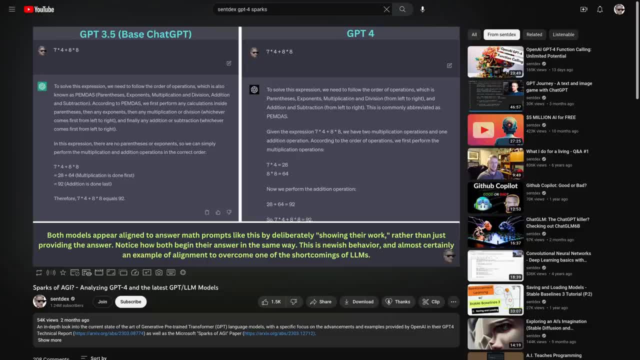 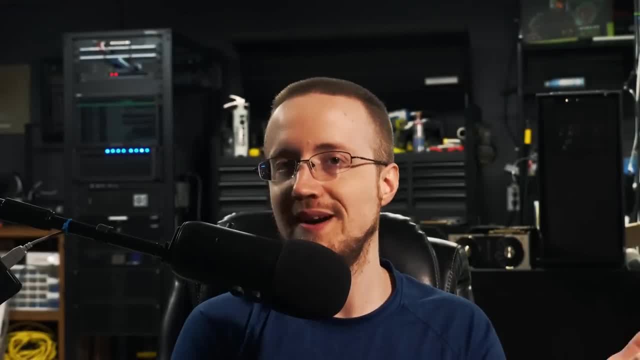 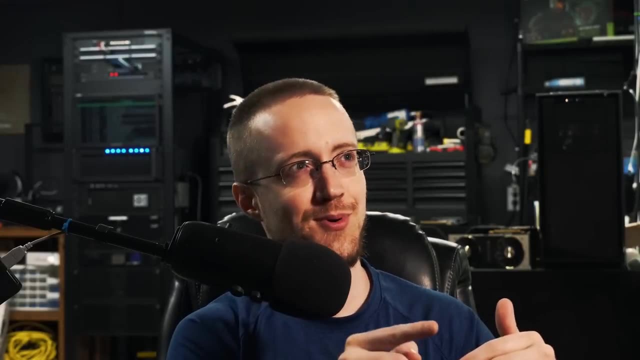 3.5. i'm just taking guesses here. but now gpt 3.5 just in a very similar way to gpt4, such that i'm pretty confident they're probably running the exact same kind of forms and like pre-pre prompts, i guess, uh, or maybe a post prompt, but i don't know how. 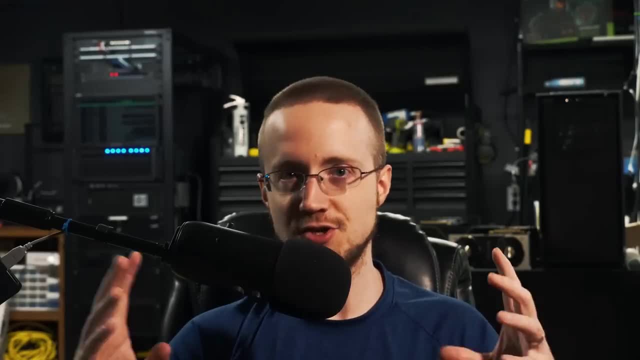 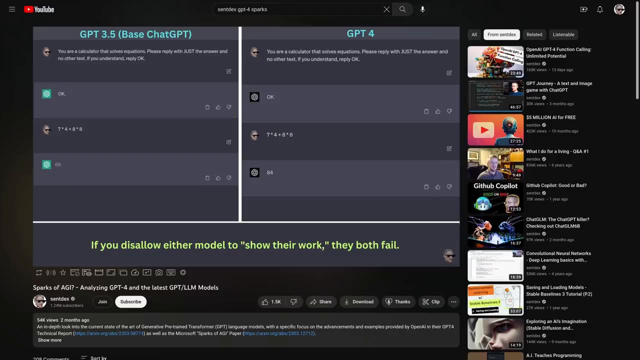 i don't know what the right word is, so i'll just call it heuristics- but essentially a trick to get the model to think through- uh, the answers. but you can still show that they will. both of these models will fail if they try to just generate just the answer and nothing more. but coming back to falcon, 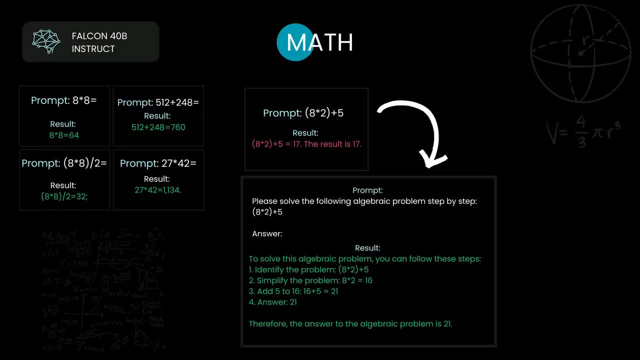 we see that if we just ask falcon without telling it to show its work, it does get the question wrong. but if we tell falcon, hey, please show your work, then it shows its work and it actually gets the question correct. another area that some gpt models are surprisingly impressive is this concept of 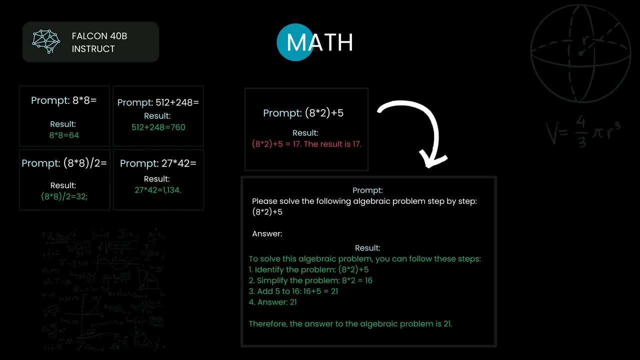 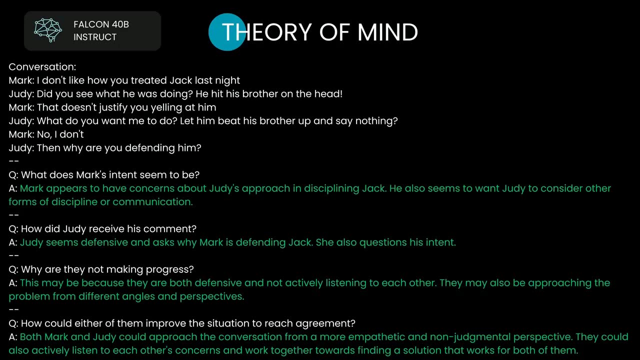 theory of mind, essentially understanding underlying thoughts and especially like human emotions and behavior for situations and scenarios. so here's an example from the sparks of agi paper from microsoft. i've run through falcon 40b. essentially the white is the prompt and the green is the generated. 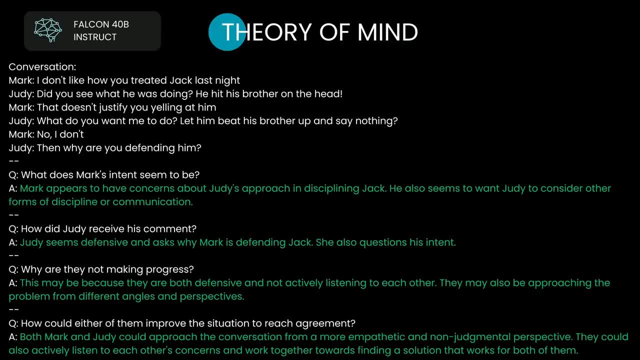 answers. i went one answer at a time each time, passing the entire history up to that point in that new question, so kind of think of this as a continued conversation between me and falcon 40b asking about this sort of conversation scenario. falcon 40b here correctly identifies that mark. 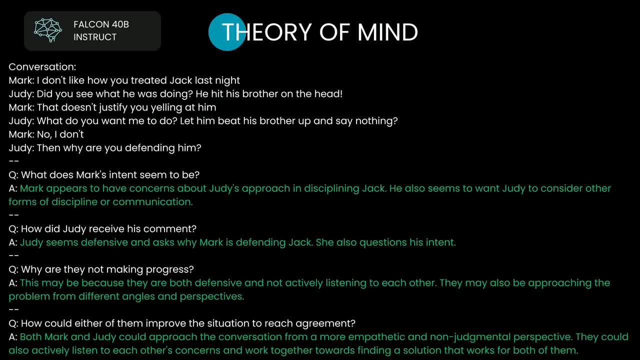 isn't necessarily unhappy with judy's disciplining of jack, but instead how she went about it but also how she's been able to do things herself and feeling about jack's sort of stepping in. and falcon understands that they're both essentially talking past each other and even has suggestions. 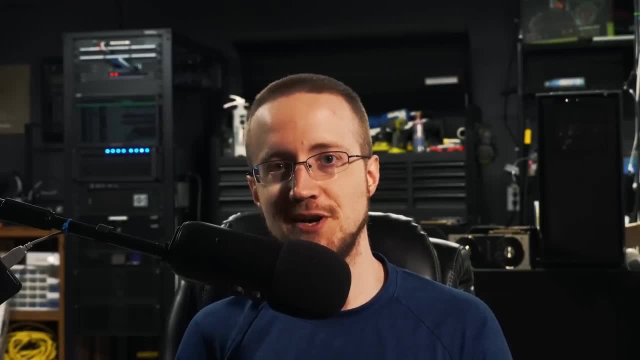 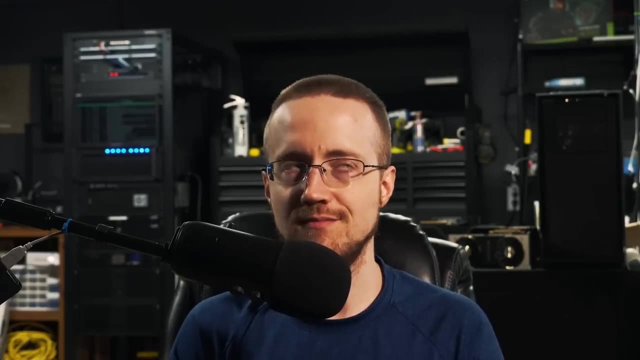 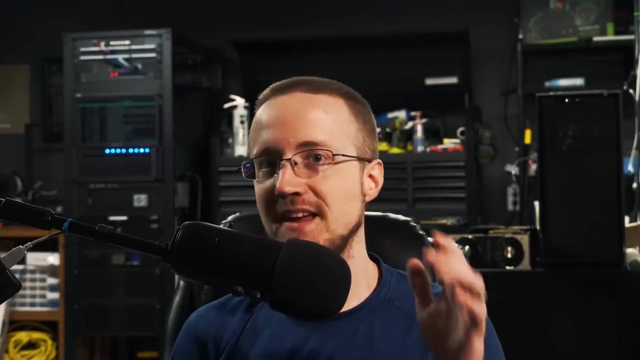 about how they could improve this situation. these theory of mind examples just always impress me, as gpt models are strangely really good at, uh, this sort of thing, often performing much better than you might have predicted if you weren't aware that these models are just good at this stuff. so 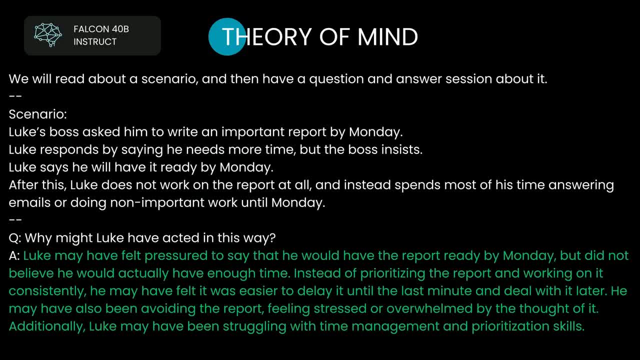 i'm going to give them a point of view now, and you can see that they're both pretty good at the same time. they're both very, very good at this stuff, and it's just a theory of mind and um an answer that i think is quite good. again, there's nothing in this text that suggests what luke's. 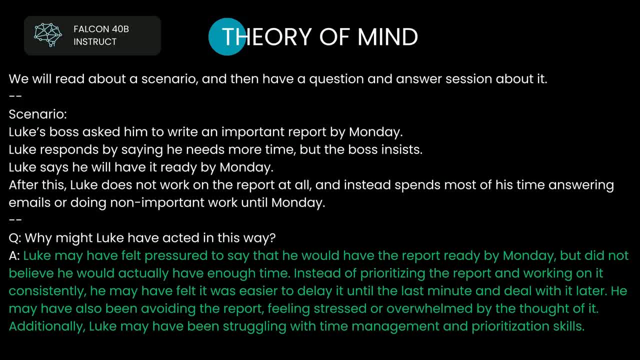 reasoning might be, this is purely an understanding of, just like human sort of psychology and emotion to attempt to explain some incongruence between requests, statements and behavior. so again, you know, generally we, you would expect ai to think in this like deterministic way and not really take into 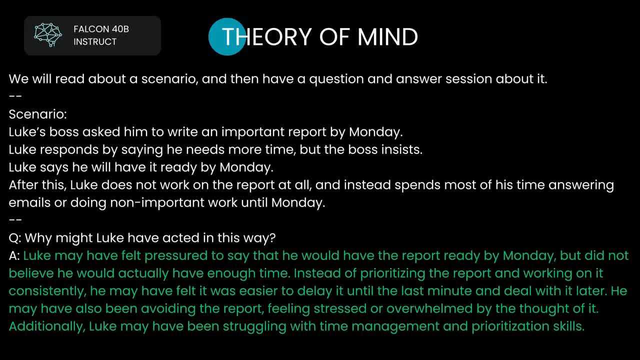 it's really just emotion. Emotions are strange in humans. It's like, as opposed to like, something like programming, where everything is deterministic and it just it's logic, right, There's this whole other side to like humans that is sometimes very difficult to understand, Whereas the GPT models 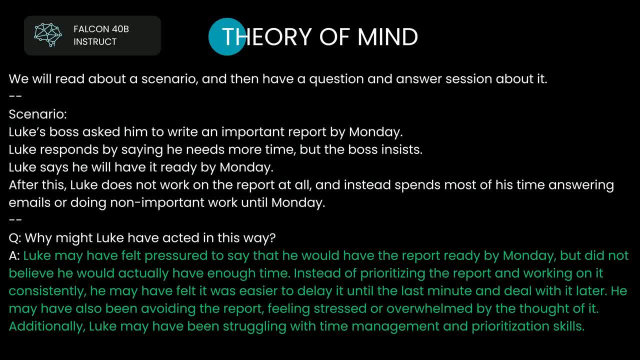 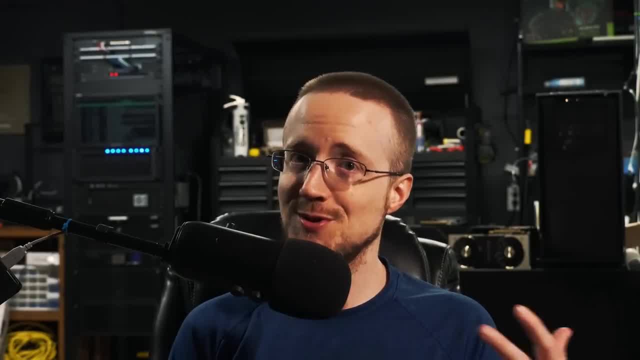 and Falcon 40B here in particular show a pretty good understanding of human emotion and behavior. Next we have some programming examples, which is usually my personal interest and focus with GPT models. 5% of the training data for Falcon 40B was code specifically, but another 5% of 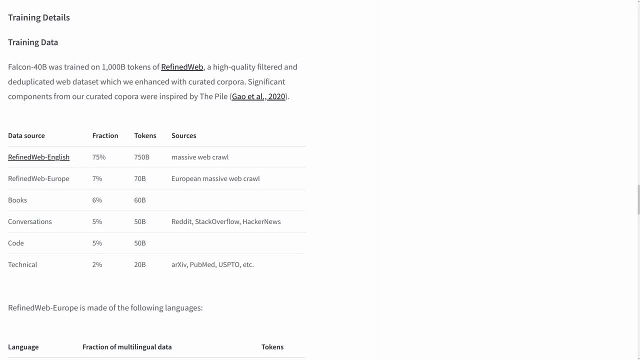 training. data comes from conversational sources like Reddit and Stack Overflow, where code is often discussed and shows up, And then there's the web crawl, which also is likely to contain a lot of code. So there's a good amount of code in here, but it's certainly not close to being. 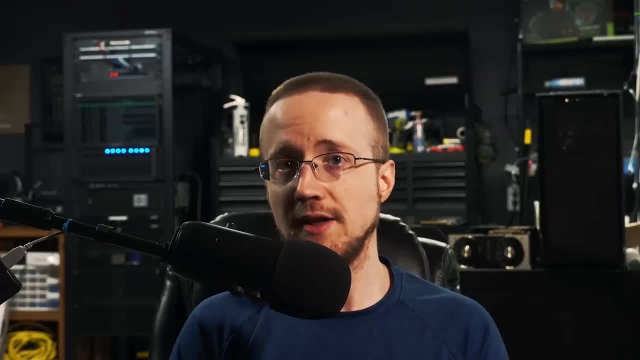 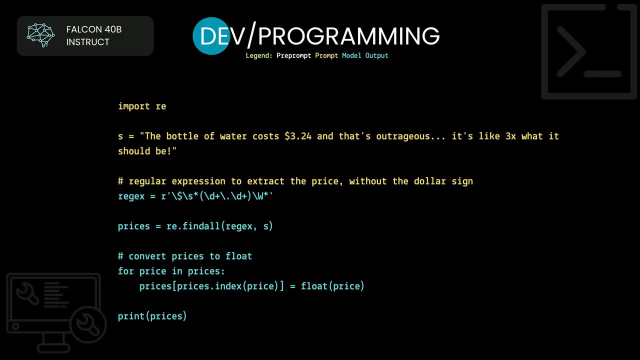 the majority. The first programming example I'll show here is a regular expression question and it's in the format of next line predictions in an attempt to simply continue the sequence, much like Copilot might do for you in VS Code. And if it's not clear, the yellow part. 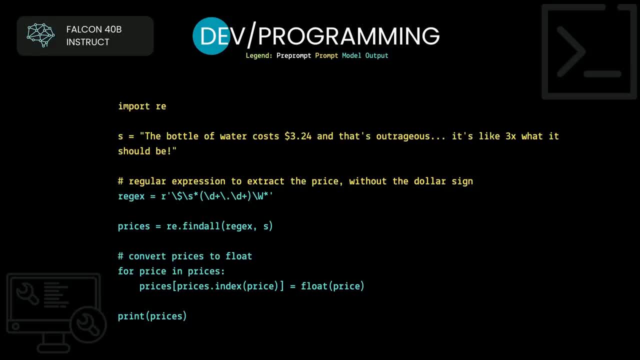 here is the prompt and the cyan is the model's output. In this case it gets the hint for my comment Again, much like I might do with Copilot, for example- and it proceeds to generate the regular expression extract the prices from the text and even print them out for me completely. 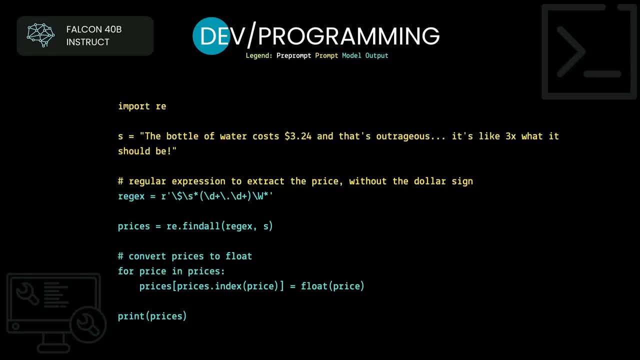 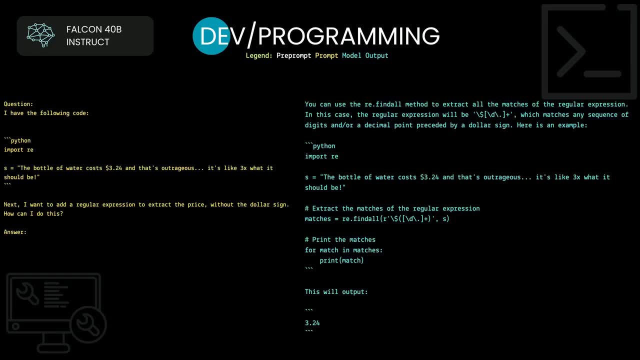 in line with what you might expect the model to generate, And this is indeed what I would have wanted. Next, we might instead enjoy a more conversational approach to the same sorts of problems. So here we've got a model that's a little bit more conversational, but it's a little bit. 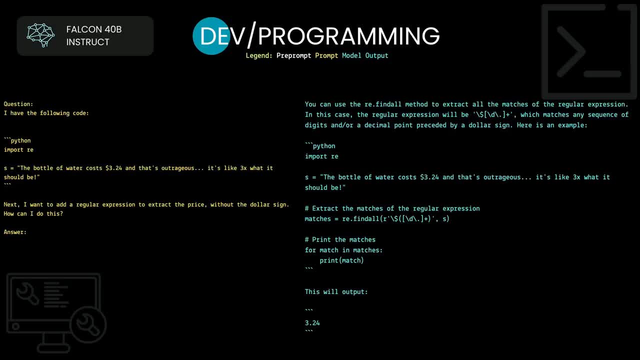 different. It's not the same exact problem, just in a more Q&A format. In this format you might prefer it purely because maybe you want an explanation, maybe from the model here, or maybe you just want it to feel more like a teacher than a code generator and give the more kind of friendly. 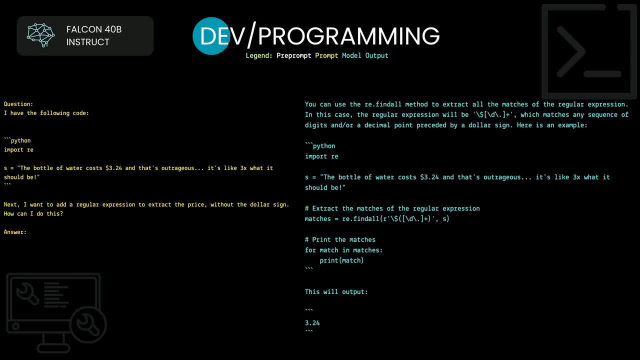 feeling to the user. It really just depends what your use case is. And here I'm just showing- and these are both from Falcon 40B Instruct, but I'm just kind of showing that you know again, you can do this, you can do so many things here. It doesn't just have. 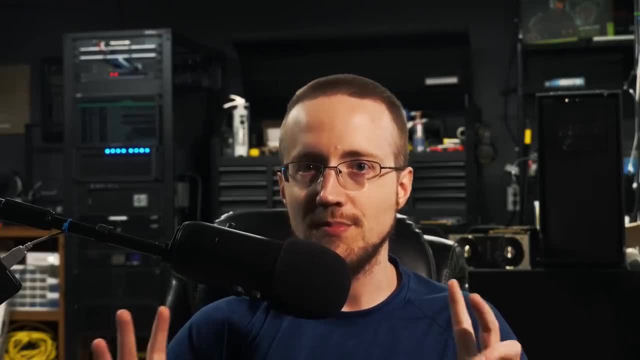 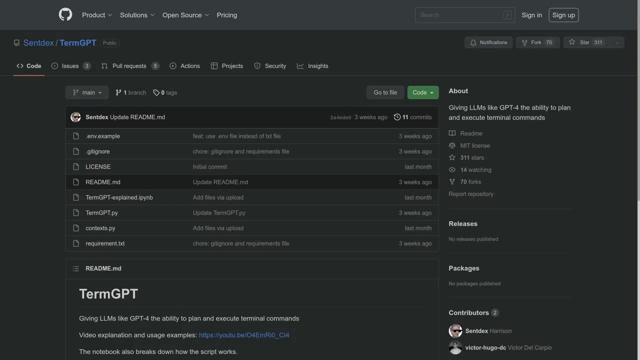 to be necessarily a back and forth, All right. so one more slightly more complicated programming example. One of my latest projects is called TermGPT, which is a project aimed at getting a GPT model to take some sort of general objective as a prompt and then output actual terminal. 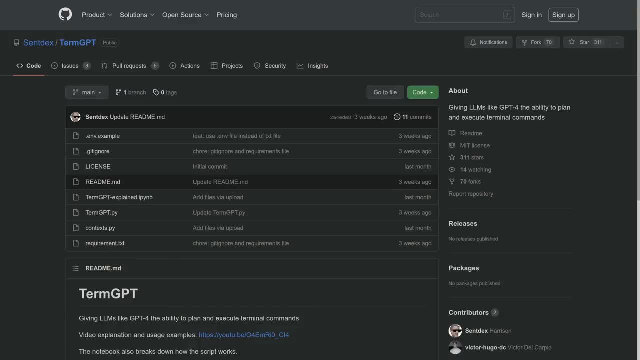 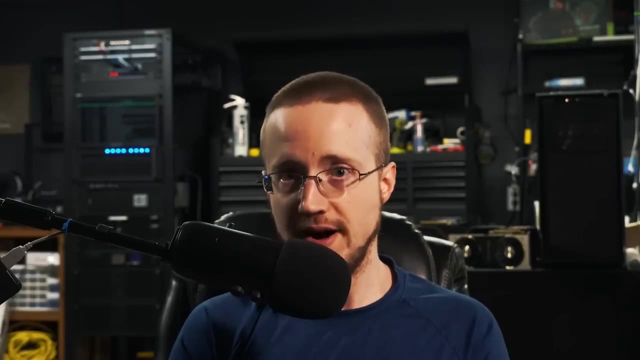 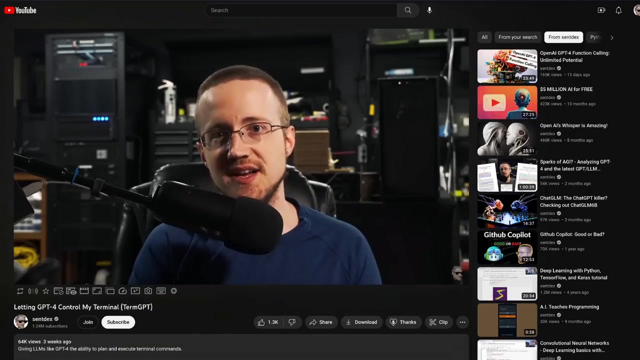 commands that could be run, even including with, like OSSystem, to actually achieve whatever that prompt was. So this includes things like, yes, writing code, but also executing commands, executing that code, Installing packages, reading and writing files, and so on. I have a whole video covering this as. 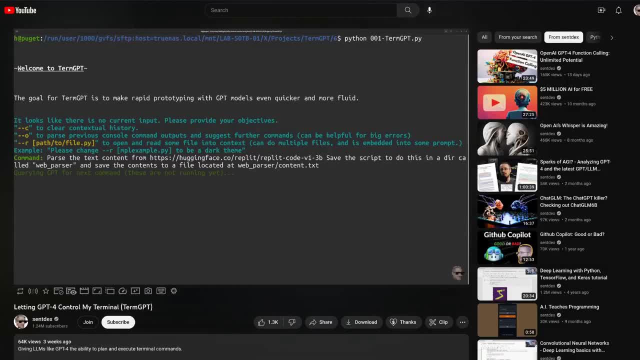 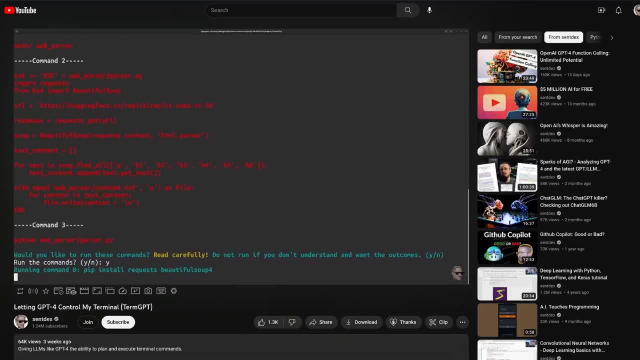 well, so feel free to check that out if you're interested. I did it using GBD4 up to this point, but I would very much like to use an open source model instead, and Falcon 40B is looking like it's- at least it's very close To achieve this with Falcon 40B, I first pass a pre-prompt with a. 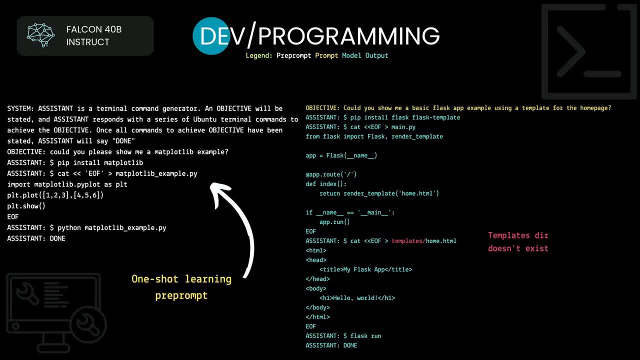 one-shot example showing just what I would like the agent to respond with, Sort of like the essentially the same thing I did with the TermGPT video, But then in this case I don't actually have to have the user specify next, because it's not required of me to do like this, like back and 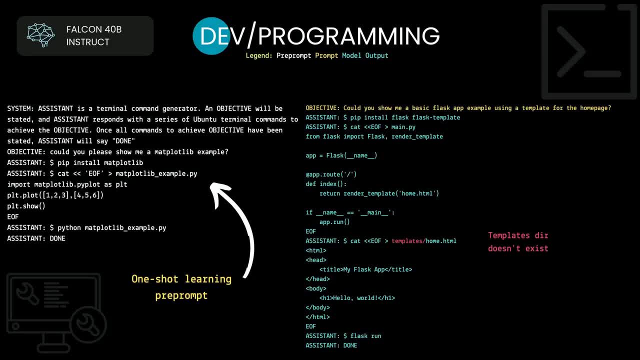 forth. So in this case I just have the user suggest an objective and then TermGPT or Falcon 40B, in this case, just suggests command, command, command, command command. So the pre-prompt shows an example of basically what I would like and then the prompt, the actual user objective here. 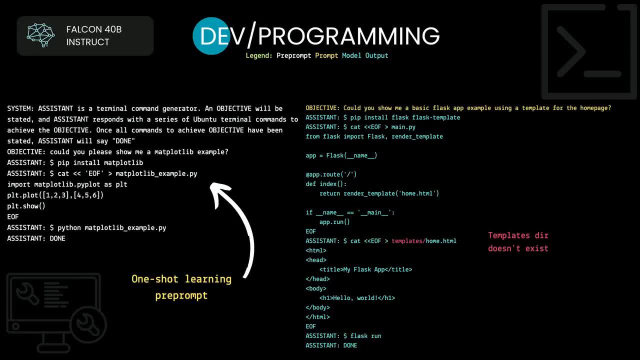 is in that yellow and then cyan is what the model's output actually was. The idea here is that a user would input that yellow part and they wouldn't even see or really be. they wouldn't know about the white part. It would just be kind of in the back end. 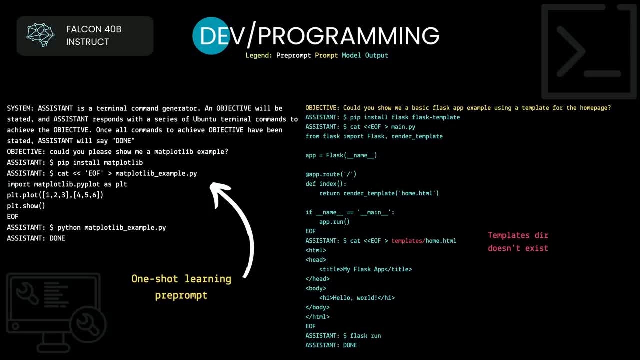 essentially. I mean, they could know about it, but they're not going to mess with that part. It's just passed there to sort of guide the model to understand how to structure its response, And then later we can pull apart that response and quite literally execute those commands. 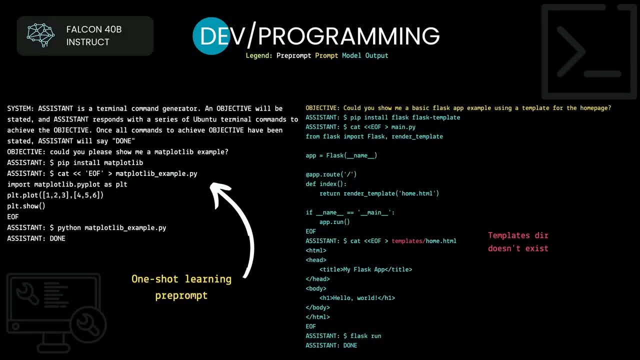 just like I did in TermGPT. So, as you can see, the output is it's so close to what we would want. It really just makes this one small mistake of trying to create that homehtml template file directory, which is correct. That is where we want it. We do want that file. We do need that file. 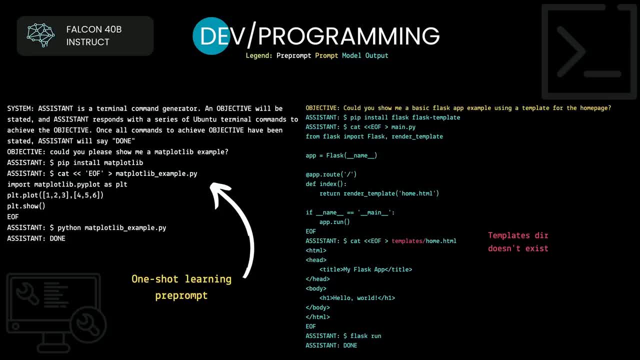 That file is correct, but we never made that directory, So in the attempt to make this file inside of that directory, it's going to fail. If we did just do a make dir that directory, this would have worked, And I think this is an example of where GPT-4 is better than Falcon 40B. 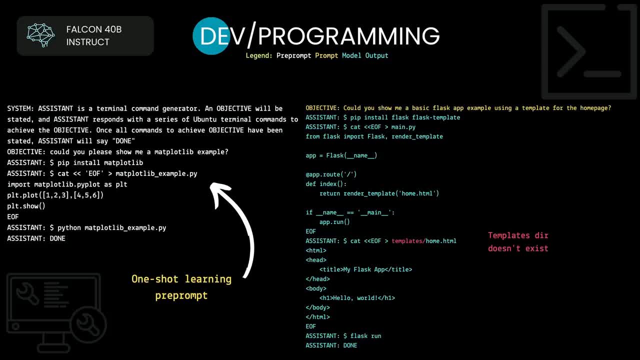 It just simply doesn't make small mistakes like this as often It can. It totally can, but just not nearly as often. And something as simple as this: if GPT-4 does solve out of the box, But Falcon 40B, at least from my testing. 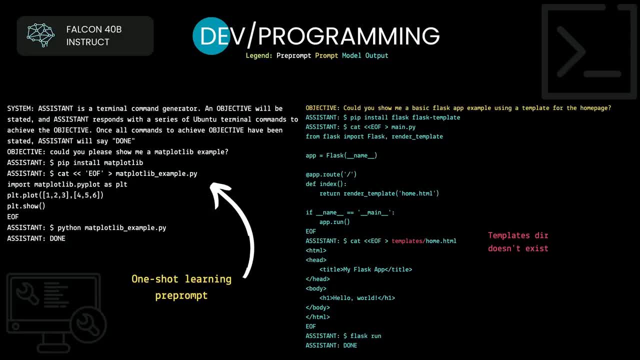 both here and just in general, I dare say Falcon 40B is actually better than GPT 3.5.. I also suspect with respect to TermGPT in general. I think with more time working on a pre-prompt I could probably iron out these problems And, for example, GPT-4's behavior has actually already. 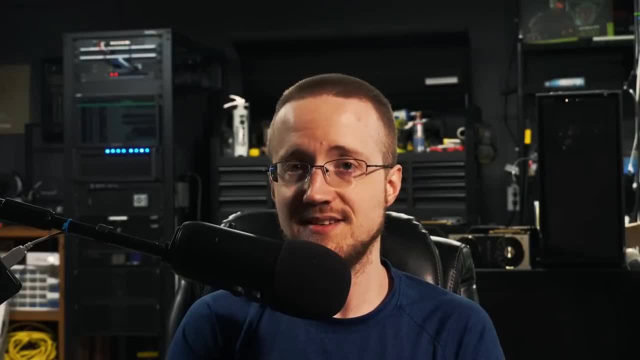 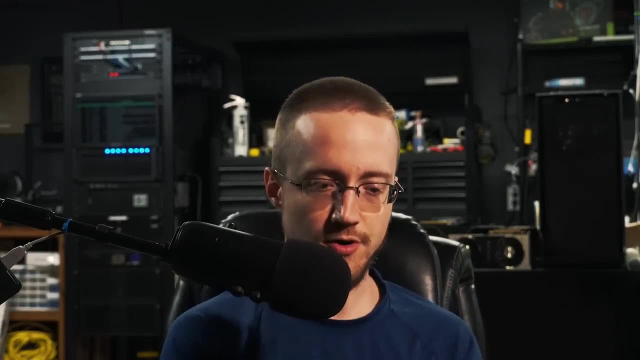 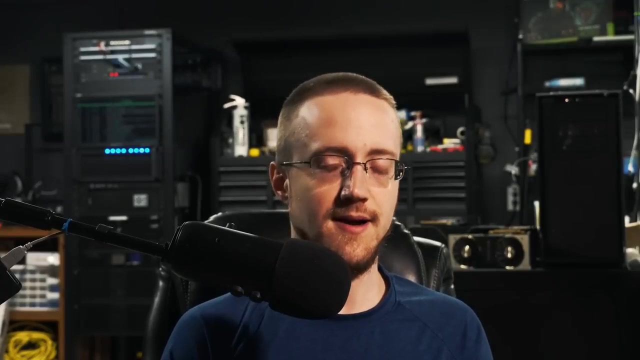 changed on me multiple times while I'm trying to develop TermGPT. Some of this is like after the fact, post-processing and kind of like double checking, And then some of that is also the actual underlying- let's call it foundational- model has also changed Now over time. that is going to keep happening And you can specify an older. 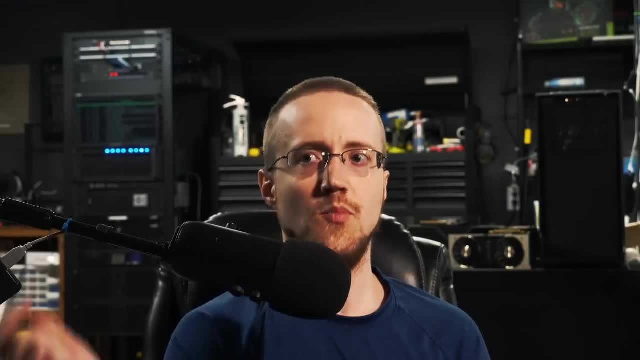 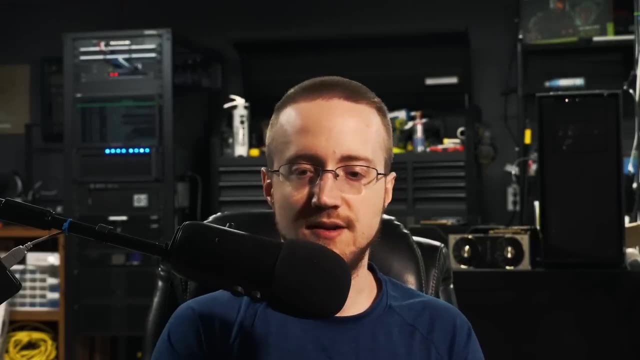 model. but I want to say they are just supporting, like the single previous model And then after that it's gone and you can't get it again. So you spent all this time really like honing in and fine tuning and getting things just the way that you want them to work. And then the model. 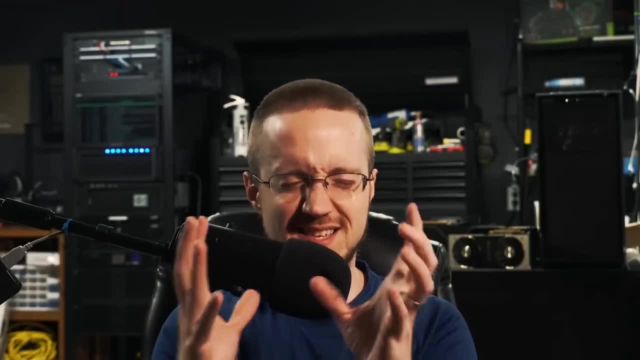 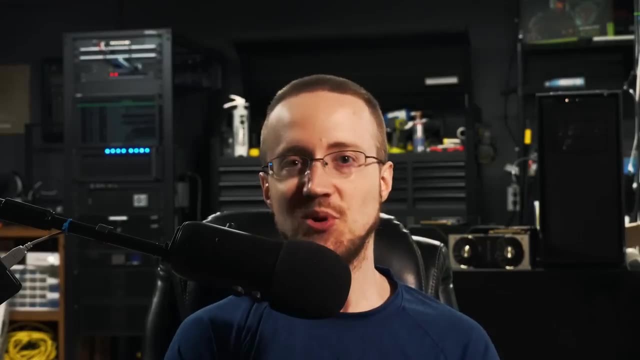 changes, or the model doesn't even change, but clearly something, something else has changed. They've changed some of that post-processing heuristic stuff and it just isn't working the way that you want it anymore And that's super frustrating. Whereas here, with this, 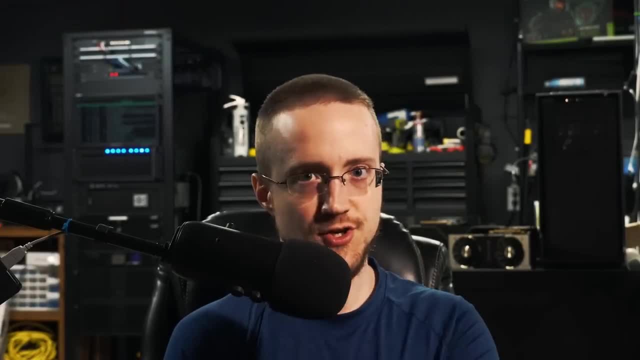 model. you can just depend. Now it's not a deter, it's not totally deterministic, but you can depend if you need it to. you can depend on those weights being frozen. They are not going to change on you in any post-processing heuristics. That's up to you, So you can depend. 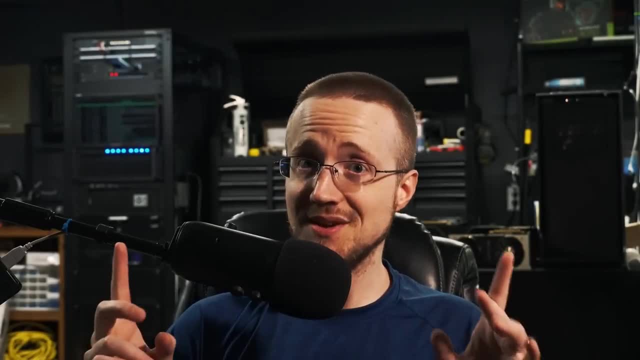 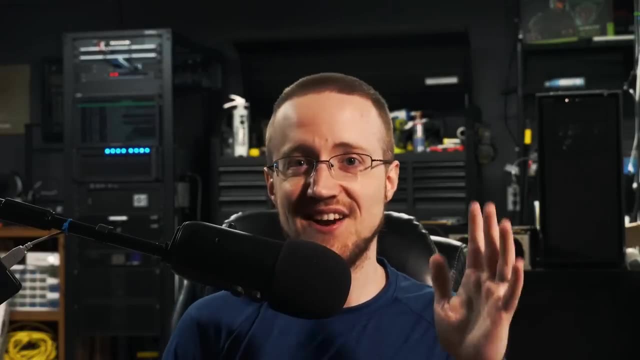 on that, stuff will not change on you. But if I want to actually fine-tune It specifically to this new use case, guess what I can actually do. that too. It's my model And I just might, like I was saying earlier, the TII or technology innovation Institute. 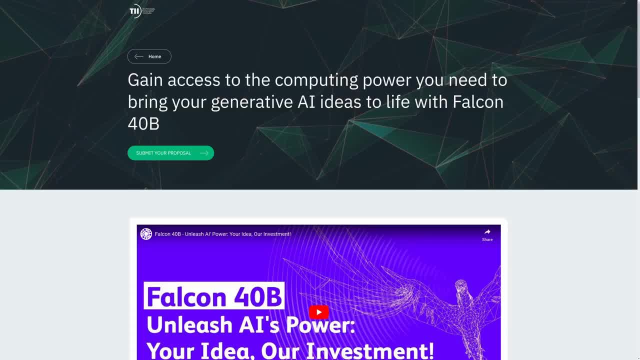 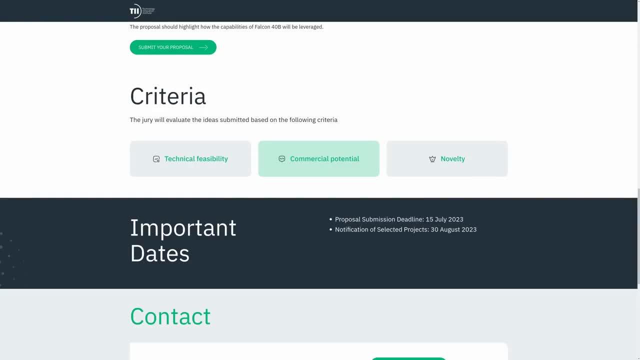 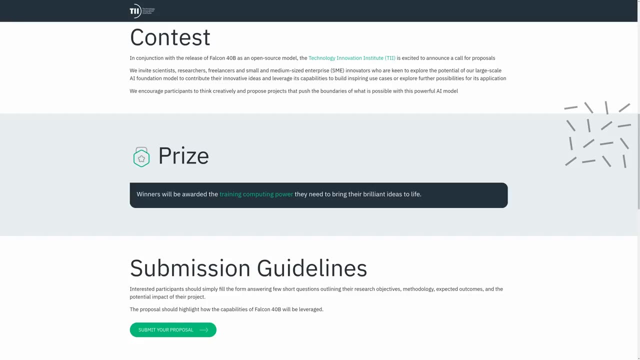 is actually currently right now has an open call for proposals for ideas that you might use on top of the Falcon 40 B model, And they're looking to essentially issue grants of 10,000 to a hundred thousand dollars in GPU compute power to people who have ideas about how they. 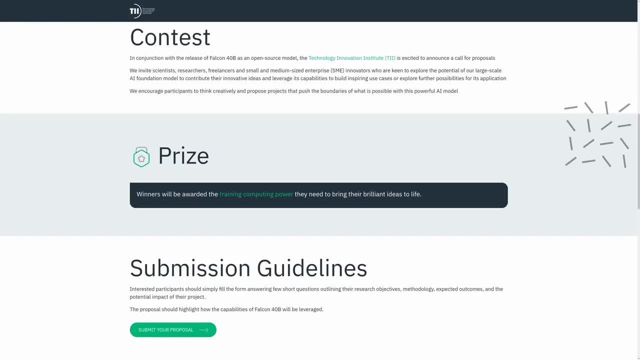 want to leverage this exact model, Something like term GPT, And I might end up submitting my own literally for that, to fine-tune it to be exactly what I want. And my suspicion is, just with a little bit of fine-tuning, I think Falcon 40 B can be better. 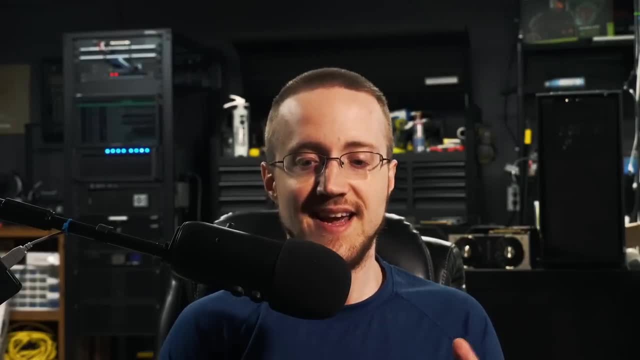 than GPT. four is right now And again. at the end of the day, it's my model. I can do whatever the heck I want and I don't have to submit my queries to open AI anymore, And I just that's pretty cool. So, with my 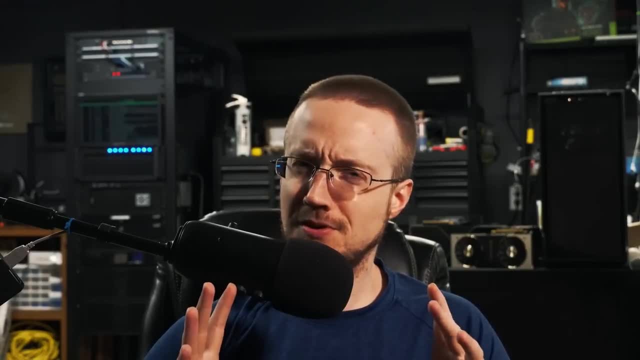 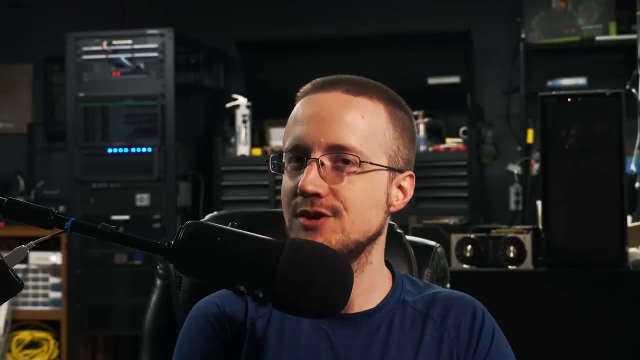 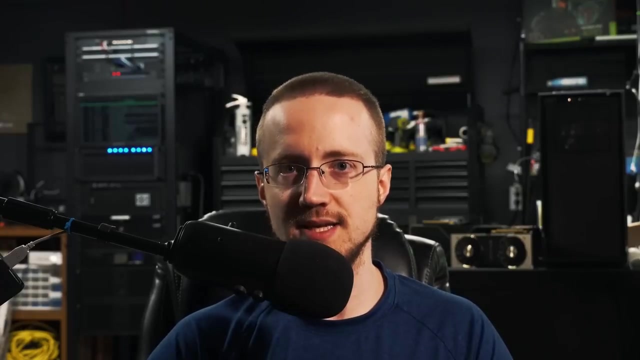 very anecdotal experience so far, I am very cautious to say, but I do think it's actually true that Falcon 40 B seems to actually be better than GPT 3.5, the base chat GPT model. I struggle with saying this purely because Falcon 40 B is such a small model relative to GPT 3.5. 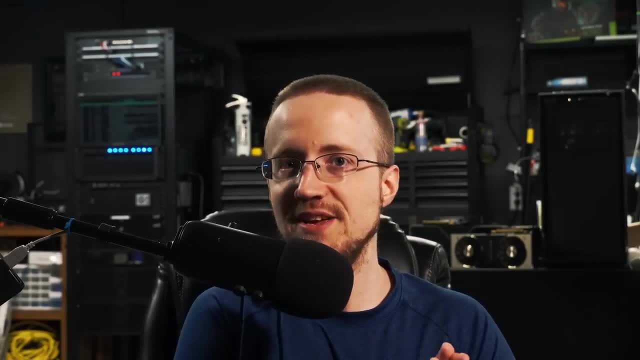 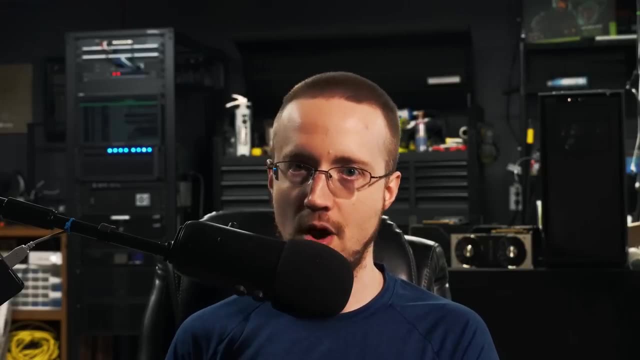 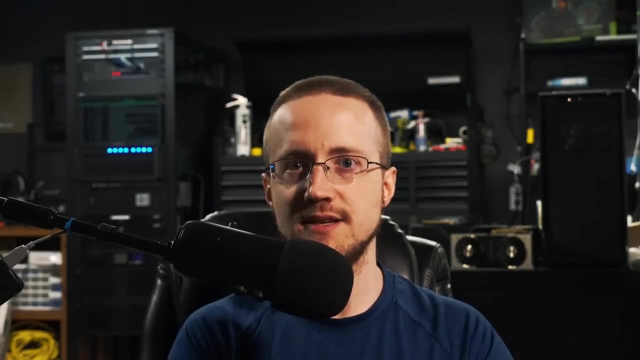 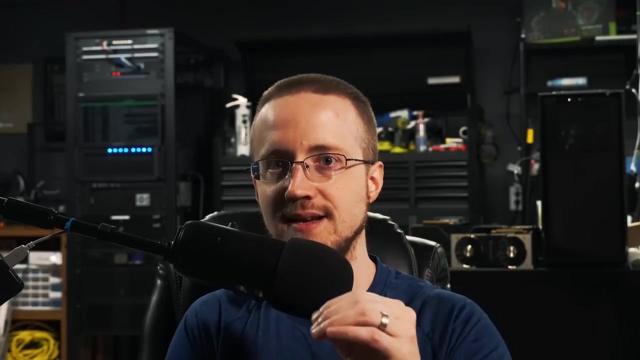 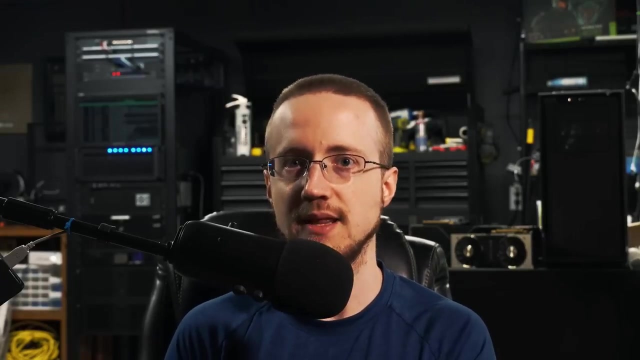 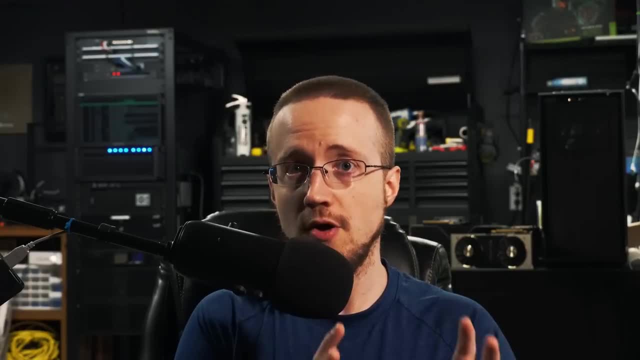 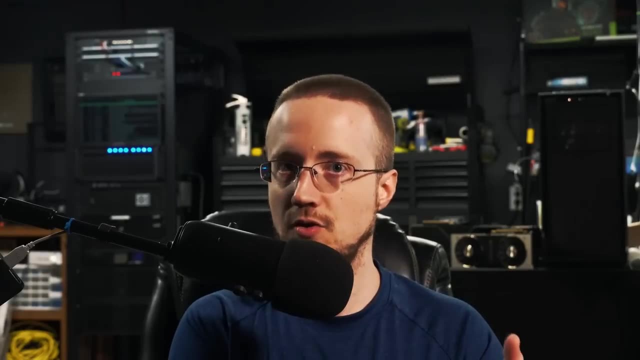 like they just are just not ideal. confident in saying the falcon 40b model out of the box is just simply not as good as the current. you know gpt4 via the api or the web user interface, but we also do know that gpt4 isn't. 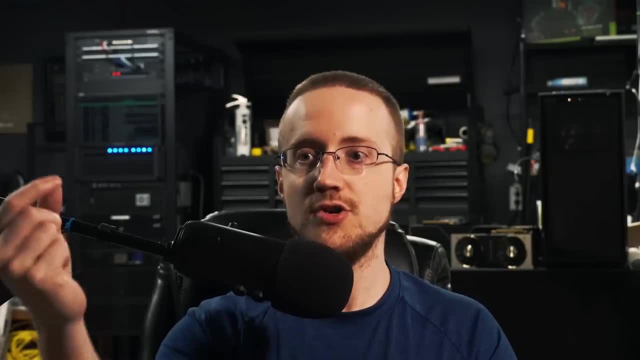 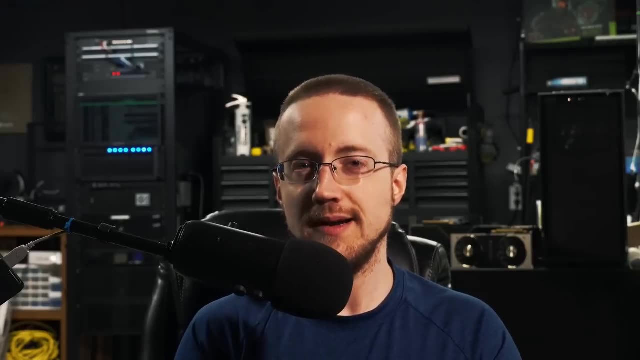 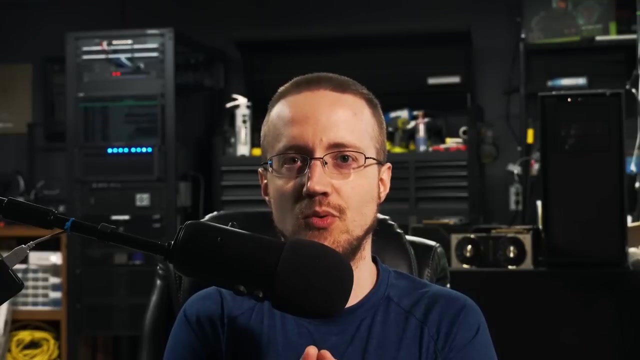 just a model like this. it's a model with a bunch of heuristics on top of it to make it quite powerful, and rumor has it that it's actually more like eight, 220 billion parameter models, essentially in an ensemble, or something like that. we we know and have some ideas about some. 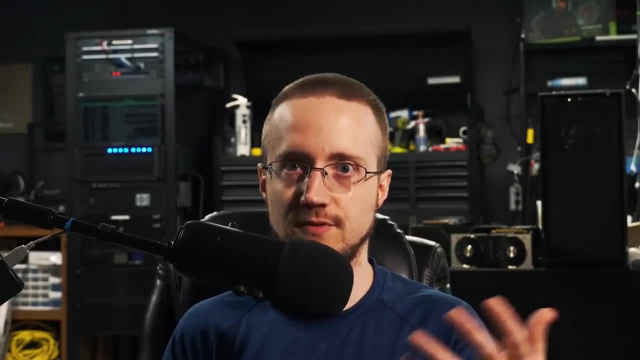 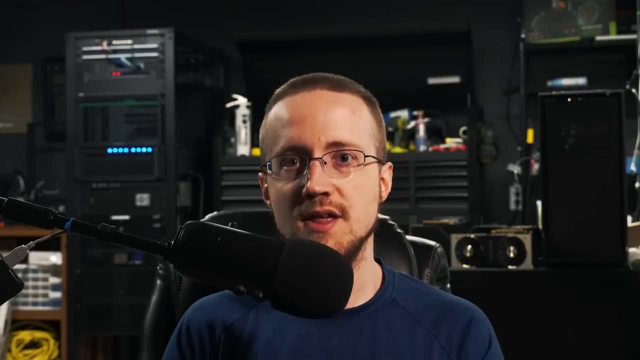 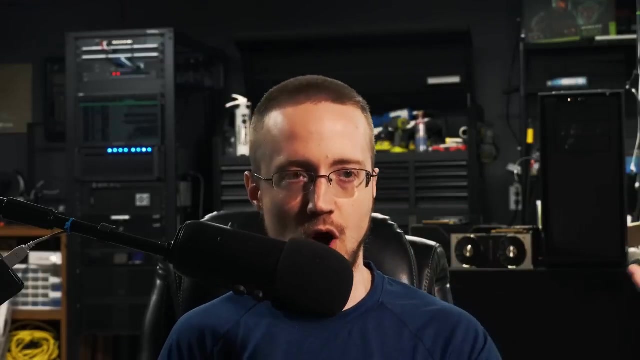 of those heuristics also used from like the rbrms, for example, that were shared in the open ai paper on gpt4. but not all and everything is rumor. we don't, we really just don't know. the only thing we do know with a large degree of certainty is that gpt4 is not just simply raw model output. 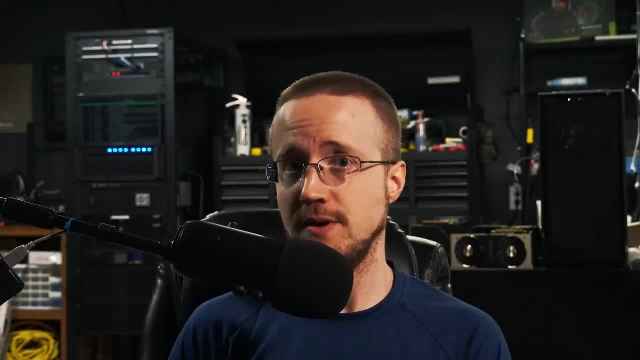 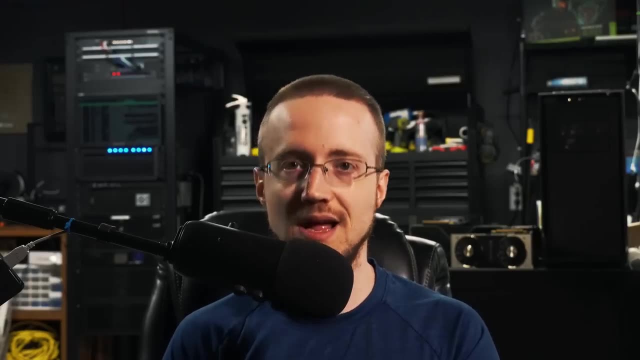 from a single model and nothing else. so based on my experience so far with falcon 40b, i would suggest that, if we like, allow ourselves to run falcon 40b with things like maybe rule-based reward models or something like that, like forms and sort of sanity checks on output and kind of. 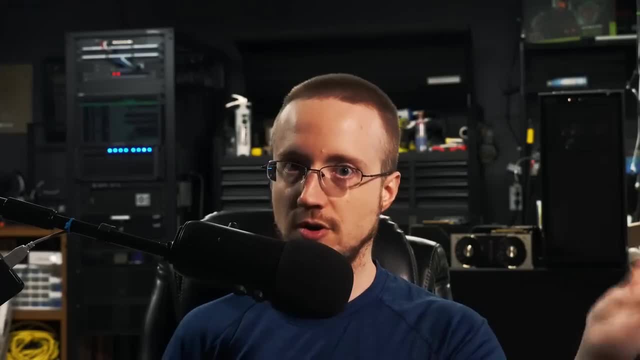 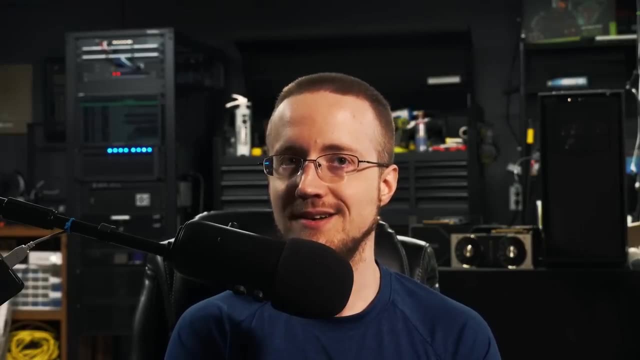 double checking or in detecting things like: is this a math problem? show your work. if so, you know that sort of stuff. um, that i think is pretty clear that gpt4 is using heavily. i all i suspect just in the response time it could be based on load, but there are certain times where you ask: 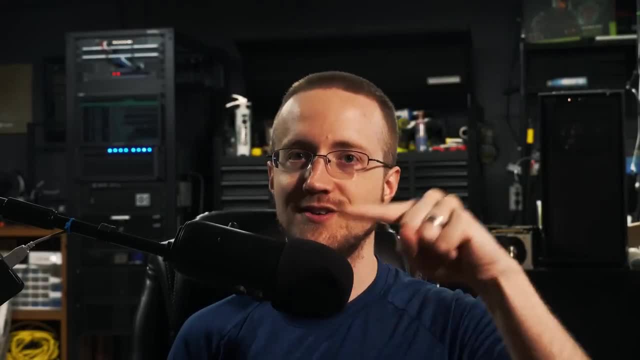 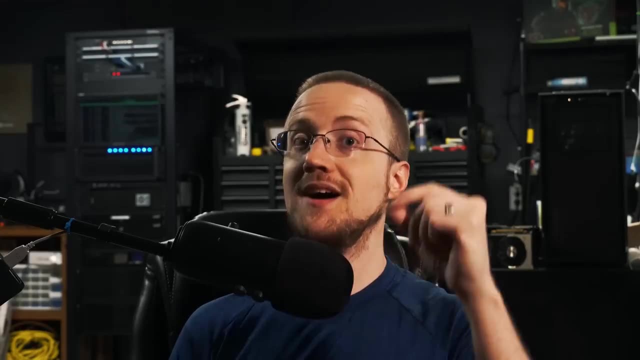 a question and you're not sure if it's going to work or not. and you're not sure if it's going to and it truly feels like you ask a question to gpt4 and you should have already gotten an answer back, but you didn't. but then you get this like careful answer back and it my suspicion again. i 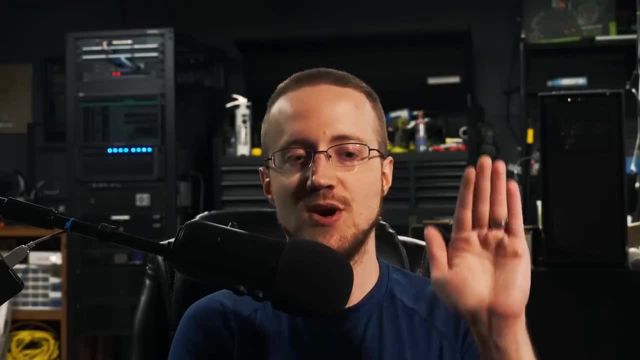 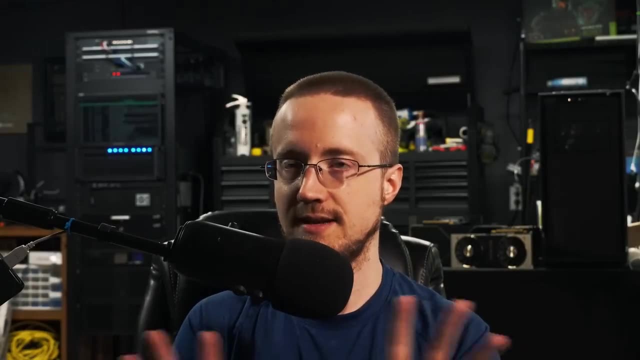 don't know this stuff, but it feels like you're asking a question to gpt4. it probably generated an output and then there's another model that sanity checks that output and if there's something that it detects as possibly problematic, it sends it in like a form with a bunch of questions and 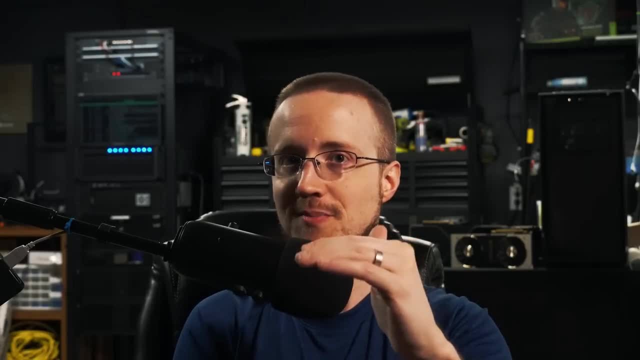 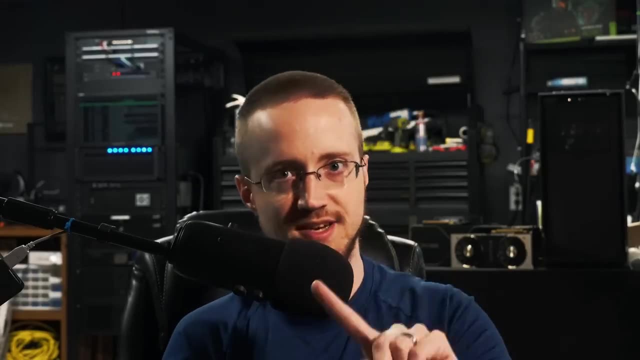 the model literally answers those, answers those questions and maybe changes the response a little bit. so my best guess is: the gpt4 model sometimes gets queried multiple times from a single user query. um, and i again i think if we, if we did the same thing with falcon 40b.